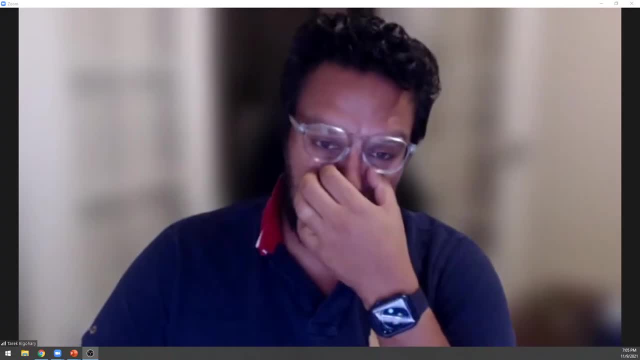 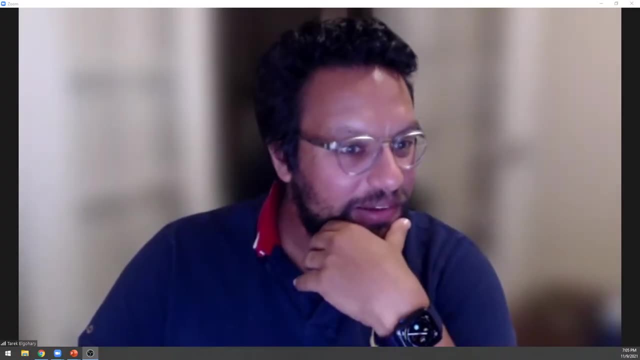 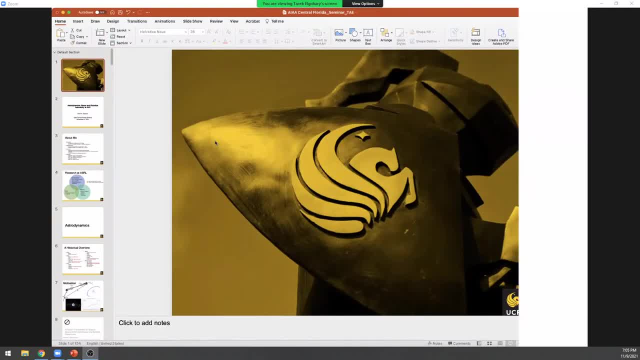 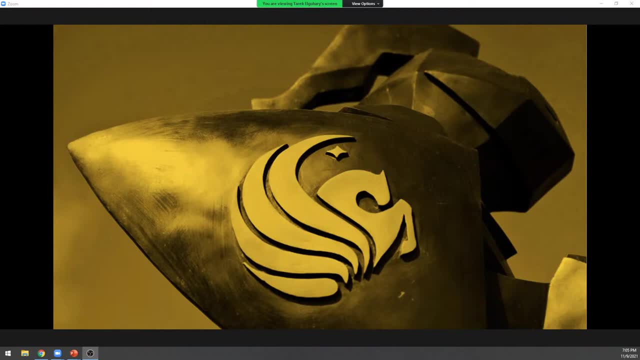 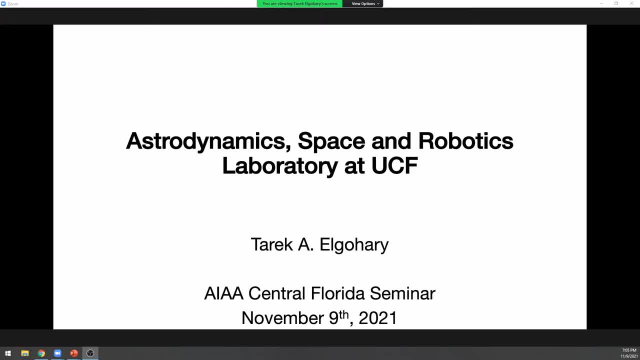 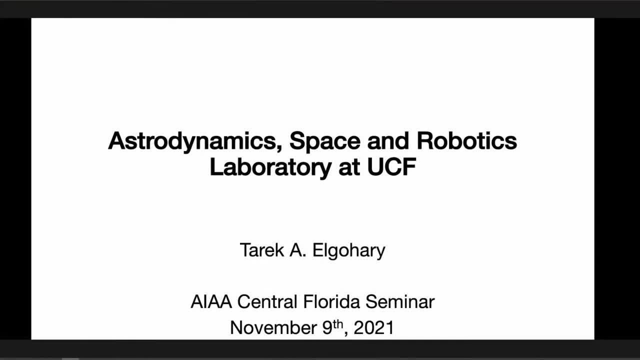 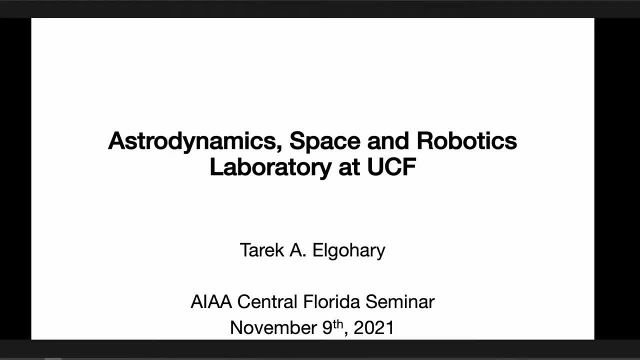 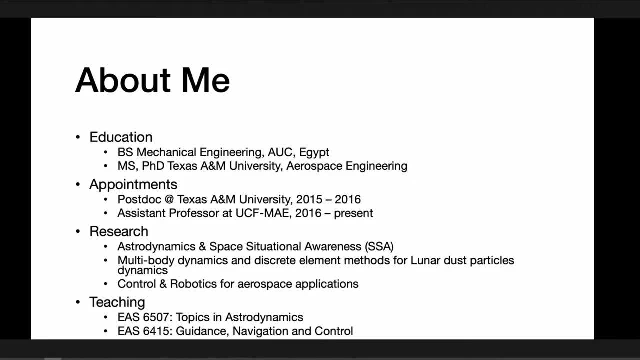 it's hard to put all of that stuff in in one hour, to be honest. so but i'll give you an overview of what's going on on my lab. a little bit about me that. i graduated with a bachelor's in mechanical engineering. then i got my master and phd for in aerospace engineering. uh, i did a year of a post. 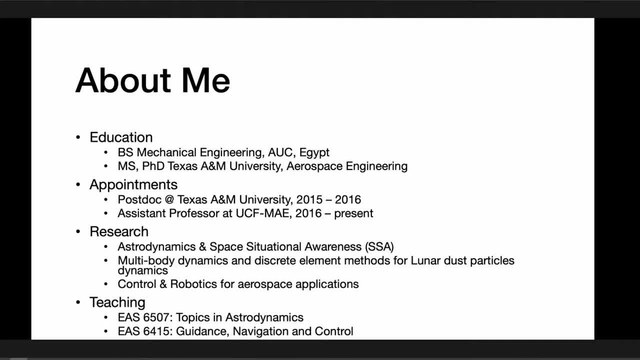 doc, and then i became a professor and assistant professor at ucf since 2016.. uh, as i said, the research areas that i'm working on are astrodynamic space, situational awareness, multi-body dynamics to lunar dust and, finally, controls and robotics in aerospace applications. some of the courses that 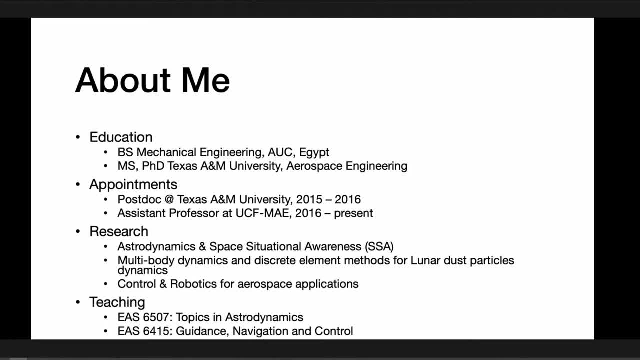 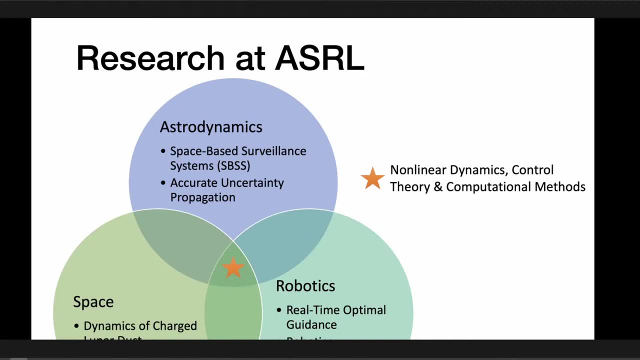 i taught were obviously astrodynamics: status, navigation, control, vibrations, control, dynamics and control, uh. so that's a very quick overview about what i do and about myself. so the this picture: it shows basically the three areas that we're working on in my lab and, although they might 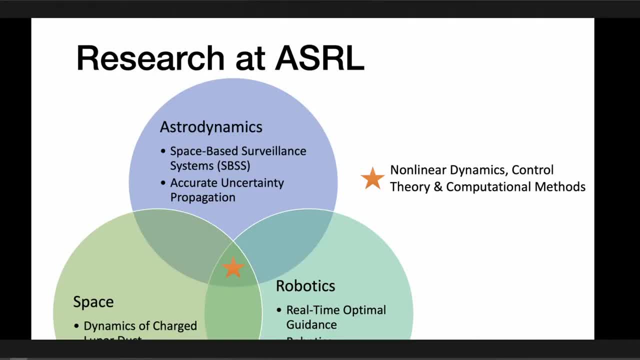 look a little bit, uh, disconnected, but they are actually all connected through non-linear dynamics control and computation methods. so in astrodynamics we're looking at space-based surveillance systems or space-based orbit estimation. we're also looking at accurate uncertainty propagation techniques. those two have elements of guidance, navigation, control as well as computational. 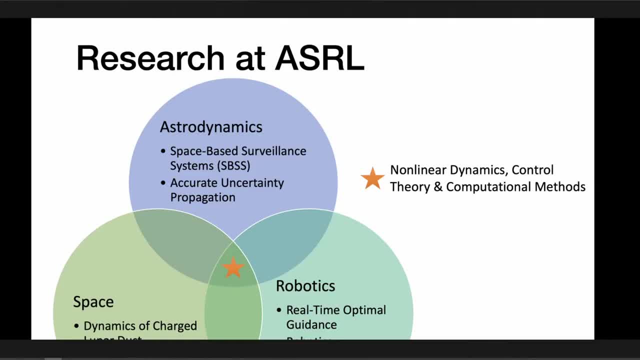 techniques for the space portion of the research which mainly focuses on dynamics of charge, lunar dust on the uh. basically, it revolves around looking at multi, multi-body dynamics and using spec, you know, a specific set of computational techniques, to solve these problems, model and solve these problems. and finally, the controller, robotics is related to 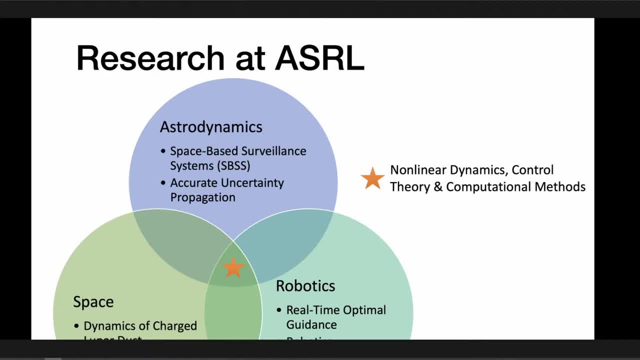 has a portion which is related to real-time optimal guidance and another portion is where we do hardware experimentation for various space applications. so the the common denominator in all of these is the research we do in nonlinear dynamics, control theory and computational methods, and that is sort of what holds all of these seemingly disparate. 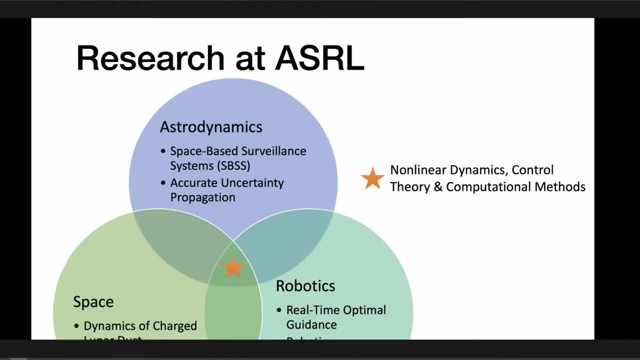 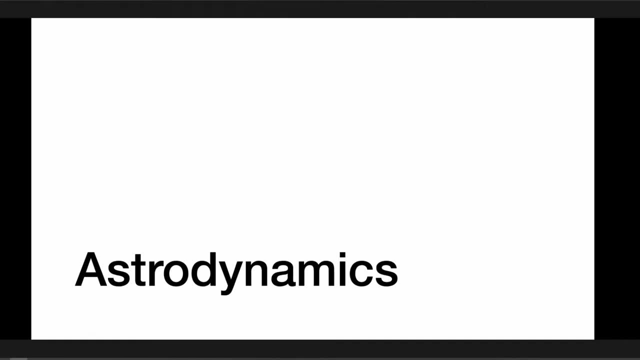 research topics together. so i'm gonna give most my talk about the astrodynamics research process, astrodynamics research going in the lab, and then i will give an overview, a little bit of an overview, about uh, the other two areas where we have uh- lunar dust dynamics and uh optimal control, and 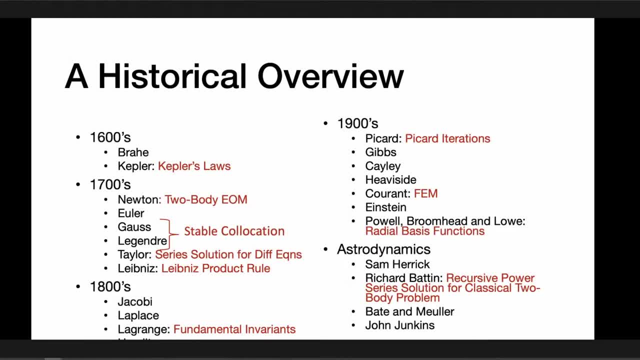 robotics and uh. this is just a a quick historical overview that i give in my classes, and some of some of the audience here are my students, so they probably have seen this before. uh, so that's a quick overview of the history of celestial mechanics, or astrodynamics as we know it. 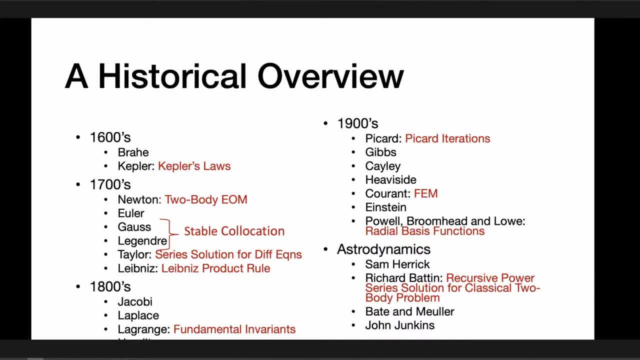 now, uh, several contributions, the main ones. you probably heard some names like kepler, newton, euler, lagrange and gauss, and most of the earlier, obviously, contributions were related to celestial bodies. later on, the astrodynamics came in, uh in in view, and astrodynamics described. 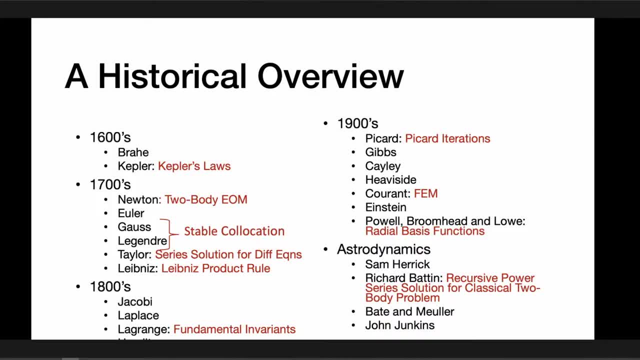 man-made uh presence in space. so man, man-made objects in space, whether it's controlled debris- because this is something we're suffering from right now- uh, controlled space flight, emissions, trajectory design and so on and so forth, and most of that falls under uh astrodynamics. several of 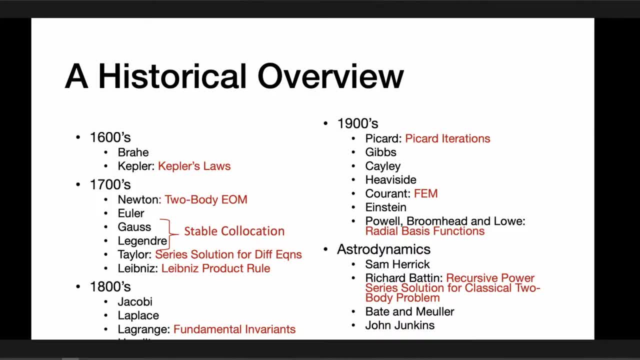 the modern or contemporary major contributors in this area is sam herrick, which is my advisor advisor, and richard beckham, who passed away four or five years ago, and that and mueller and then my advisor, jean john. so those are main areas of, or main people that work in in this area of astrodynamics. 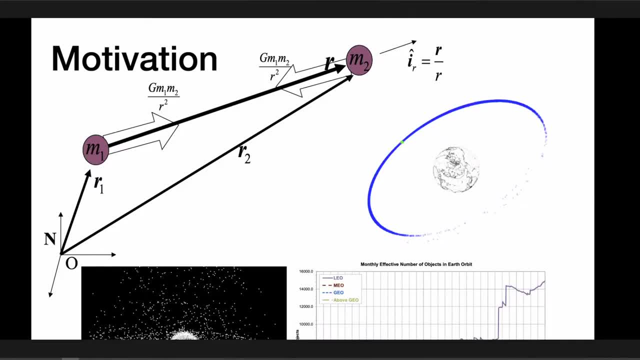 the motivation behind doing research in astrodynamics is sort of a coupled problem of an increasing debris population in the various space orbit, and these pictures below are basically from nasa space debris. we basically track space debris and you can see there are some events that took place due to collisions or experiments that caused a jump. 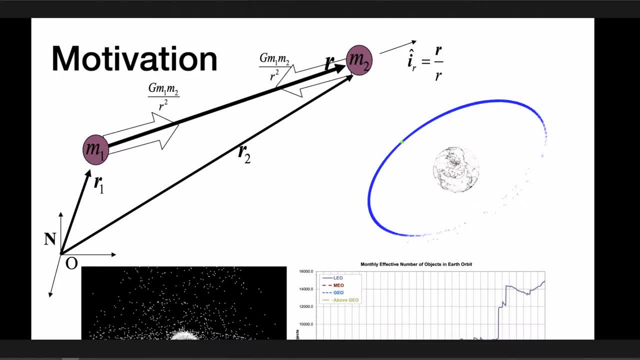 in in the debris population. now there is a theory out there that's called kessler's syndrome. that says that more debris will collide and disintegrate, causing more debris to exist, so essentially an exponential growth in debris, the other part of that problem. so we have here what represents. 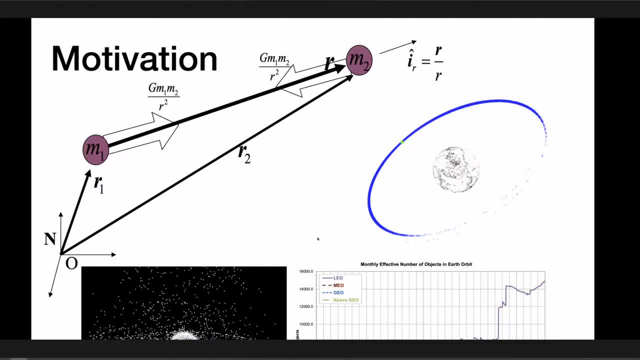 an increasing population in space debris and potentially, as you can see here, the you know the, the plots, it shows an increasing trend in the various states, the various earth orbits, whether that being more debris, more dramatic in Leo orbit, but it still exists in the various bands of Mio and Gio as well. 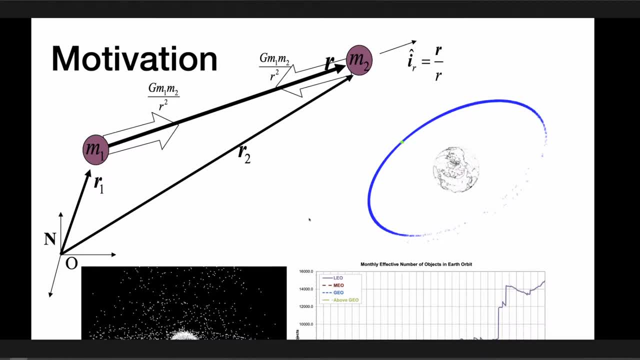 And, as I said, the fact that there is something called Kessler's syndrome or Kessler's theory, is that these objects will keep colliding with each other, producing more objects, with a prediction of exponential growth of debris. The other aspect of that problem is that the two-body problem, or the governing equations, which is part of the 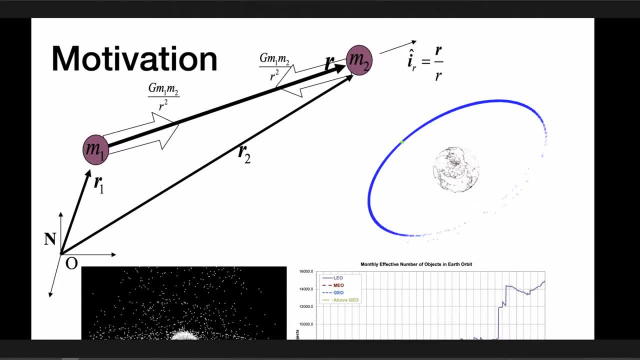 nonlinear dynamics aspect of the research we're doing is essentially a nonlinear problem, highly nonlinear problem, with several perturbations, Just the two-body problem here, and this is, you know, what describes the interaction between two masses and distances between them, you get this inverse quadratic gravitational law that we all know and love. 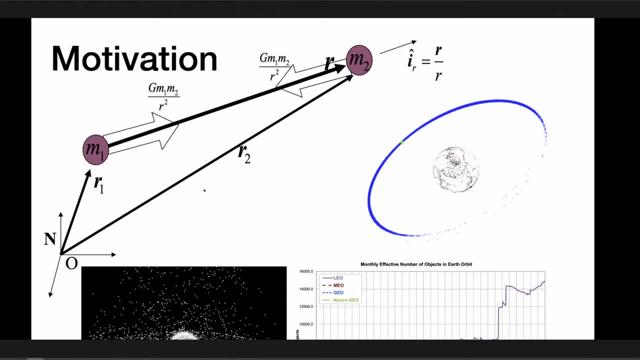 and also, on the other hand, uncertainties because of the nonlinearity of the problem. if you started with this dot of distribution, of initial distribution of particles after one orbit, this is the distribution you get after one orbit around the earth, and this is without including any. 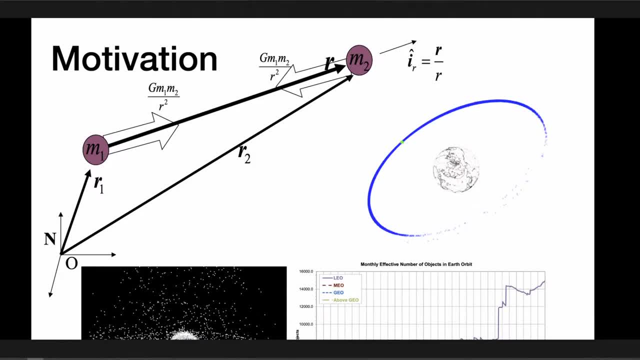 perturbations or even uncertainties in those perturbations. So the orbit problem is nonlinear by definition and it basically affects the propagation of the uncertainties as we go forward in time, and that's why we are studying these problems where we're developing. 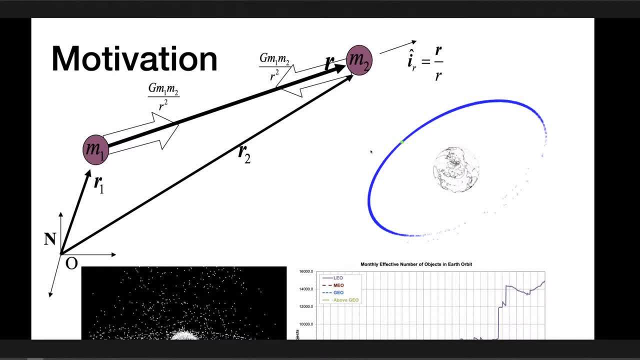 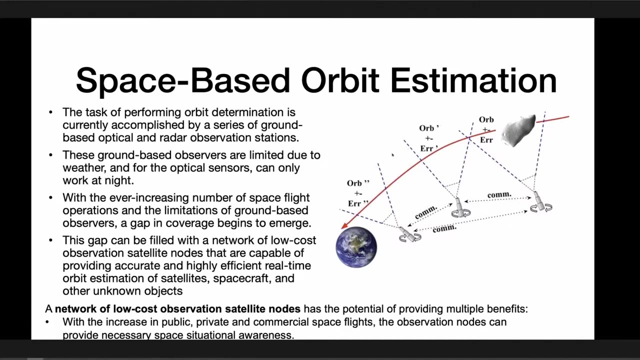 methods to: number one, better identify objects in orbit and number two, how to essentially propagate those uncertainties accurately so that we get better orbit predictions, in the absence so of measurements. So the first aspect, or the first part of this would be related to: 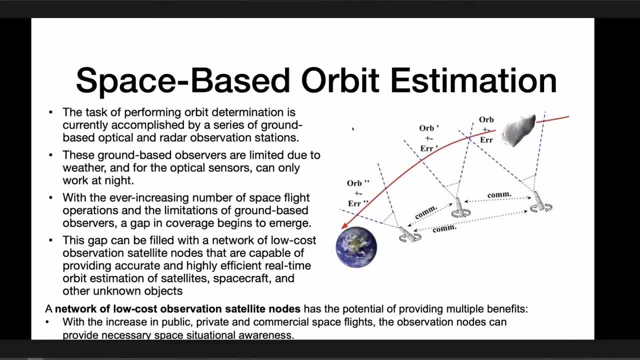 space-based orbit estimation. Now, the current state of the art or the current approach of doing orbit estimation is this: there is the space surveillance network, which has several ground stations and a very limited number of space-based observers. This is basically managed by now. Space Force. 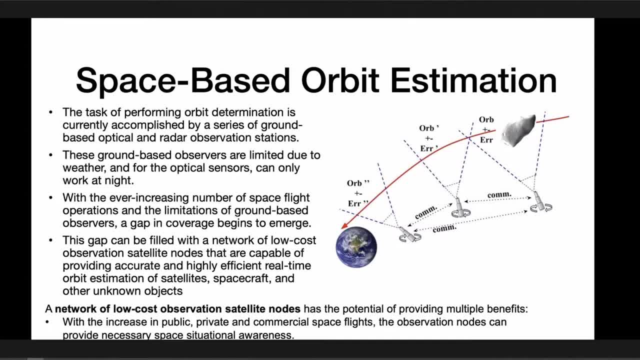 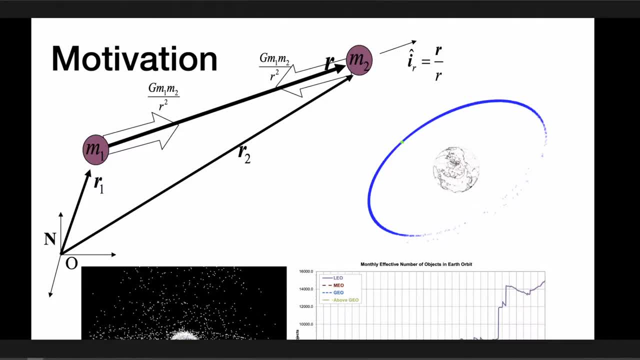 and essentially tracks all objects, not all objects like that population of objects. Now this is about 20,000 objects. if you added all of them up together, you're talking about 20,000 objects that are trackable. These are usually about 10 centimeters in diameter, so a size of a baseball. Populations that are. no one knows, to be honest, the actual numbers of populations below that number. some estimates says we are between between one centimeter and 10 centimeters. we are talking about 500,000 objects, and below one centimeter we're talking about millions of options. So no one is actually tracking those. 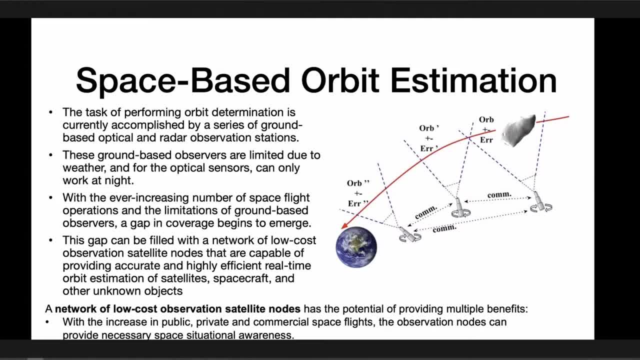 Now, if you're following the news, there has been a couple of ISS encounters with debris and some damage was done on some of the solar panels of the ISS. So it's a problem that can actually jeopardize existing satellites and can even jeopardize lives of astronauts in the ISS or scientists in the ISS. 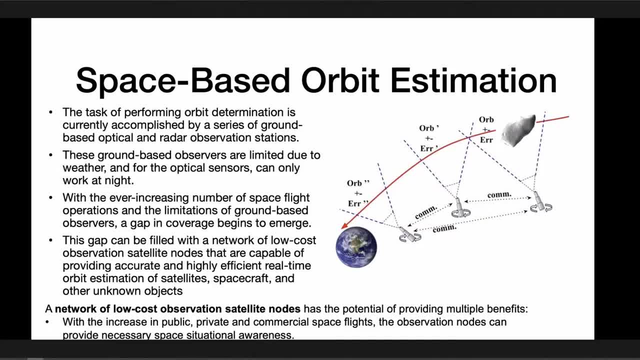 So one area that we're looking at is space-based orbit estimation. Now, this area has been looked at- and there's another name for it, called space-based surveillance systems, And this area has been looked at for quite some time And it suffered from some deficiencies- is that there is an ambiguity when you, when you take measurements in in space. 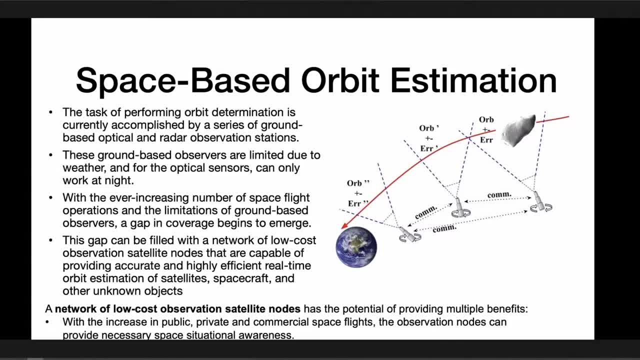 without range, like if you're using a camera, you get, you don't get range information. And if you don't get the range of information, this problem- there is a problem about it- introduces an ambiguity or, in other words, an observability problem of the object. 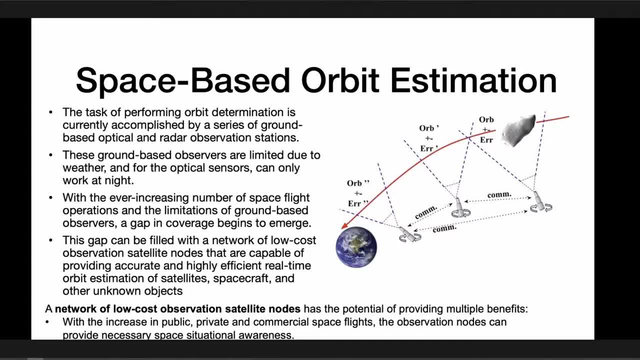 which essentially affects the estimation. Now this has been tried to be resolved several ways: using thrust to essentially modify or take measurements from different perspective, using stereo cameras and so on and so forth. But each type of camera can essentially look at a specific or each solution where we're using a specific way of measurement and there was no way of unifying all of these measurements to produce better results. 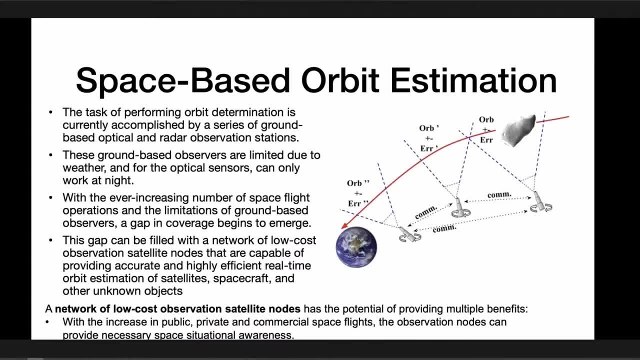 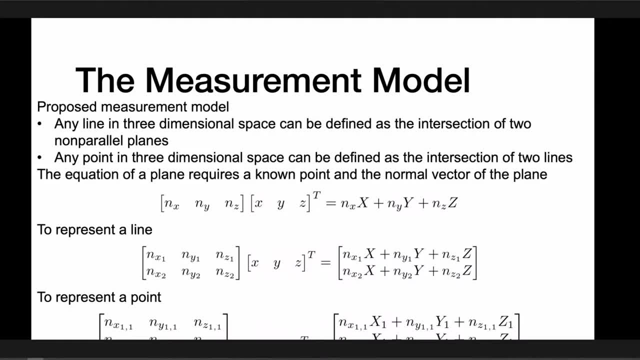 Now what we have looked at is coming up with sort of a unifying measurement model. That unifying measurement model essentially comes. it was motivated by the angles only measurements, So by monocular camera measurements, if you will, And this is where a lot of math would start. 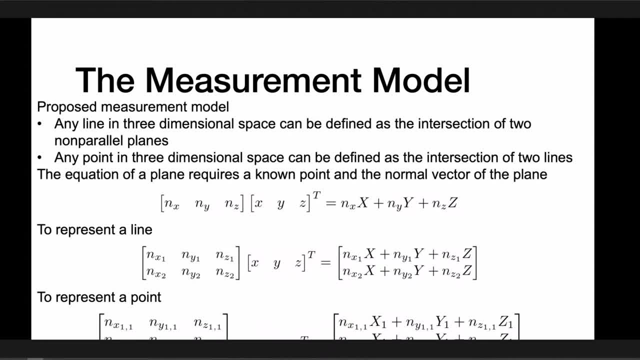 So hopefully it's not too much, But the idea- the basic idea is quite simple- is that you can use intersecting planes to define a line and use intersecting lines to define a point in 3D space. Now that, combined with the fact that you can have measurements from different objects, is what motivated- sorry- different observers, is what motivated our research. 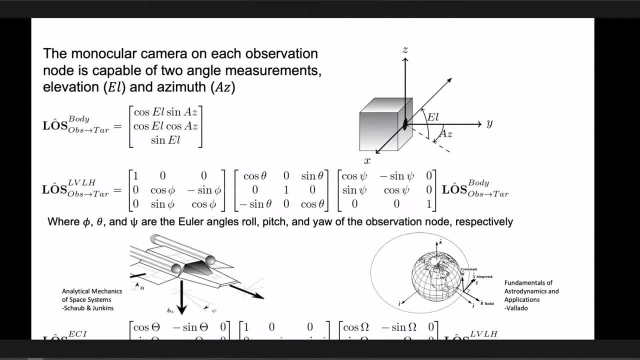 So if you look at, you know a very simple representation of an observer spacecraft which measures two angles, measured or shown here as azimuth elevation In the body frame. then you go through some coordinate transformation to move this measurement in an inertial frame. 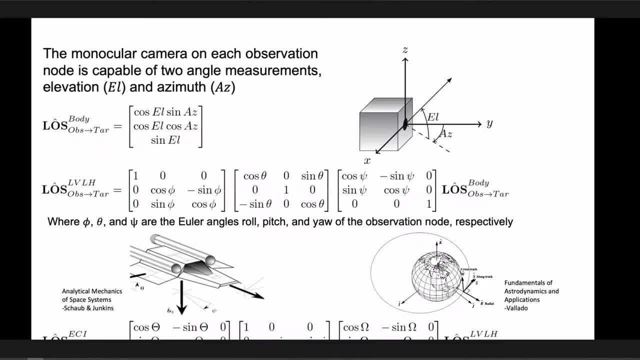 So you go through. you go from body to the orbit frame or the radial along track and cross track frame or the Gaussian frame forward, and then finally you go through to the inertial frame. So once you have these measurements in the inertial frame, you can start defining. 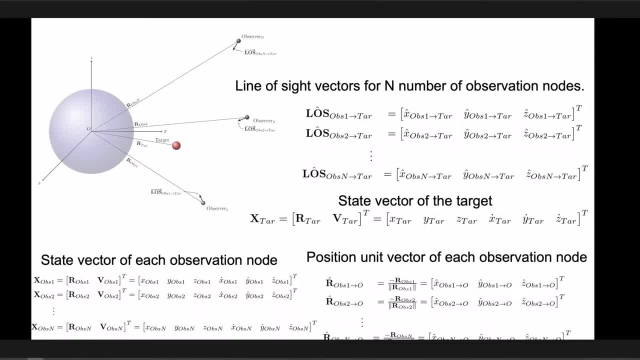 line of sight sequences, or you can start defining line of sight vectors, So one from one observer to the target, from the second observer to the target, from the nth observer to the target. these are vectors that define line of sight or that represent line of sight. 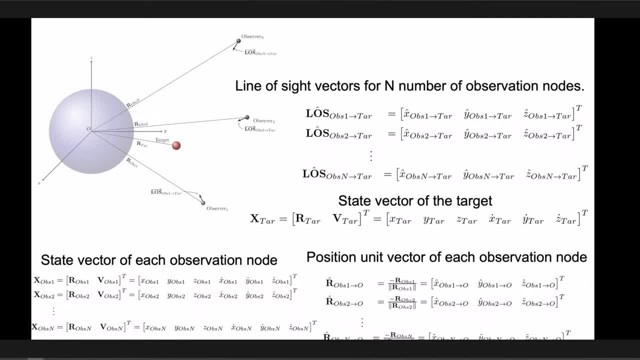 Using that line of sight vector, you can represent the. there is an assumption, obviously, that we know where the observers are, We have certainty In the position of the observers, And then we can essentially define the observer unit vector from the zero, which is the inertia frame centered in the Earth. 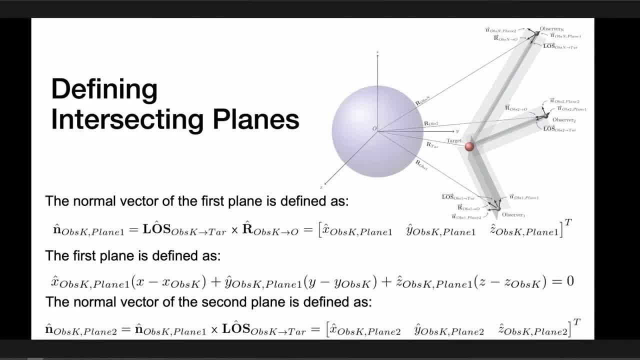 and observer one through observer n. Having those set of vectors, we can start constructing planes. So remember, the original idea was that we need to do intersecting planes, but we need to construct intersecting planes, and then we construct intersecting. 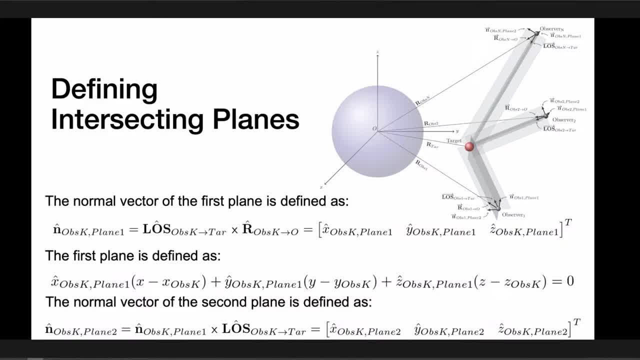 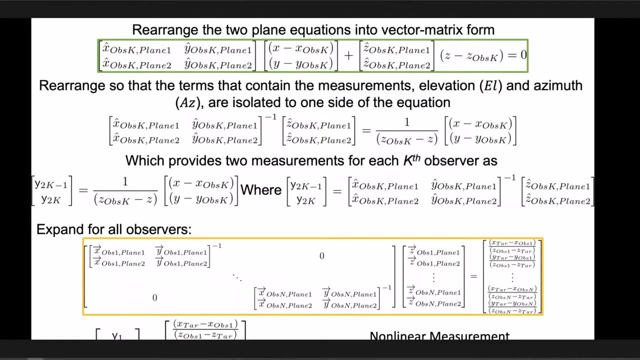 from this we can construct intersecting lines so that we pinpoint the target in 3D space. So first we define a couple of intersecting planes and we essentially start to look at their intersection. And what we can end up with after some rearrangement is this: 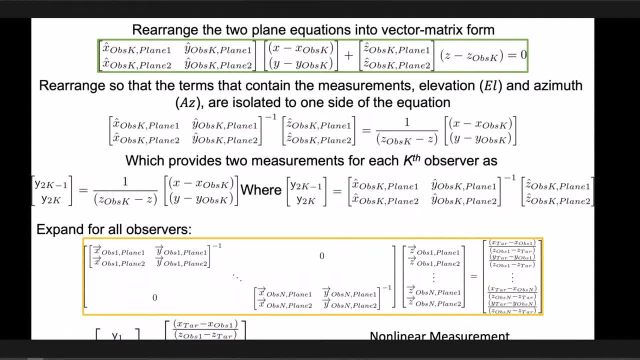 matrix in this yellow or yellowish orange box, which essentially represents the input from each separate observer unit. And this is the input from each separate observer in a measurement model that looks something like a measurement. y is a nonlinear function of x, x being the unknown state of the target. 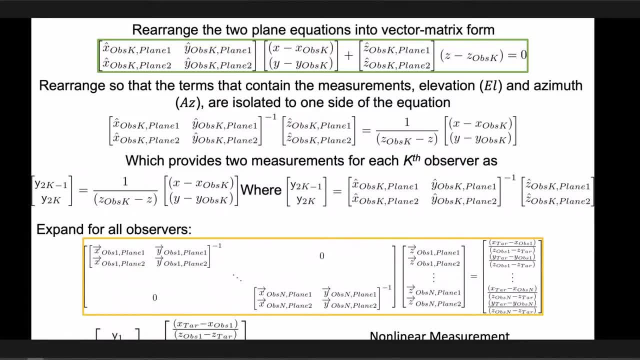 Now I'm showing this structure. this structure, because it's it's quite important in our idea, is that once you have the structure, it doesn't matter if you're measuring angles only or range only, or range and angles or any combination thereof of measurements, because 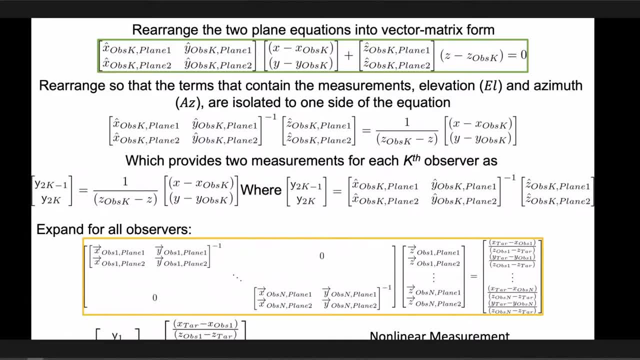 each observer contributes to that matrix by this block, sub or sub block matrix, as you see here. So now you can add and remove measurements as you see fit, depending on their availability, whether they are good or bad, whether they are of the same type or different type, or whether they are synchronous or asynchronous. 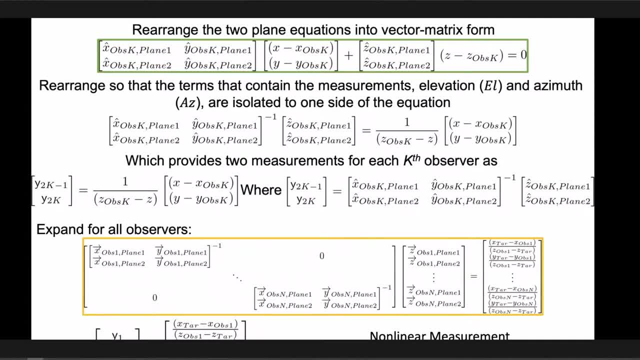 So that becomes very a very versatile measurement model that can accept or that can unify measurements taken from different observers using different senses. Here we're focusing more on angles only because that's part of the set of results I'm showing here, but the the model is quite versatile and can accept different measurements from different. 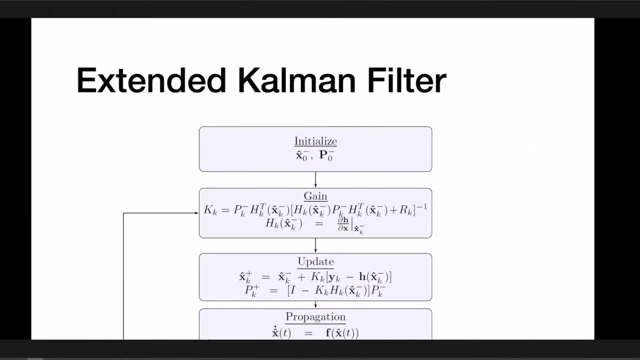 sources. Now, after you do this, you have this structure where you have a nonlinear measurement model that can be fed into a simple- for now a simple- Kalman filter. With the Kalman filter, you see, if you're not familiar with the Kalman filter, 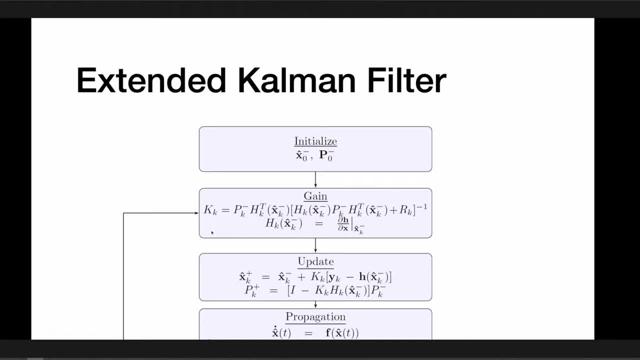 you essentially start with a guess, compute, some gain. that essentially is used to update your state and error covariance- And we will talk about this later because it's part- because this error covariance essentially gives you an idea about the uncertainties in your model. 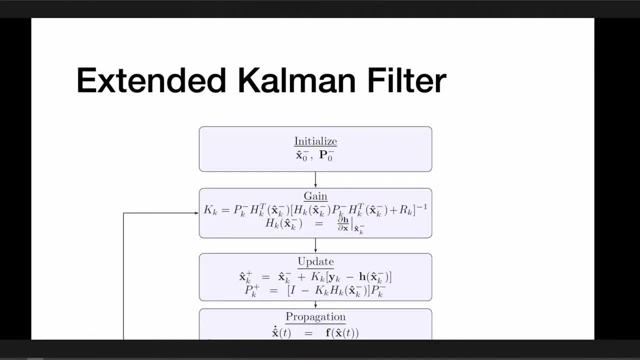 And afterwards you propagate the dynamic and you propagate the dynamics and the covariance and then recompute the gain, update, propagate. Each time you do this step is that you're inputting a new set of measurements And each time the time as time goes forward. 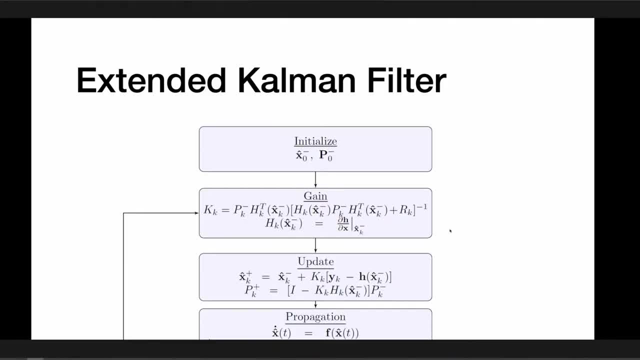 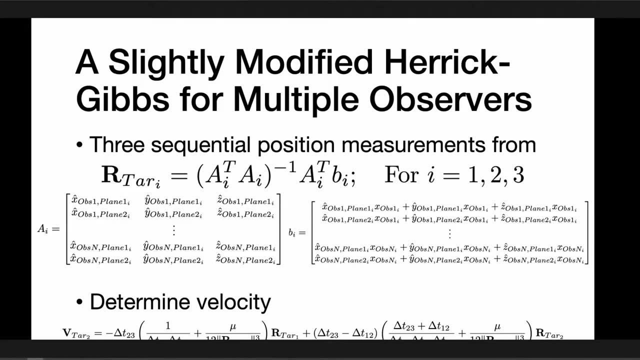 you're essentially obtaining more accurate results about the order. Now, as you see here, we have to initialize that filter And to initialize this filter we so we modified a known method for initial orbit determination to include inputs from different observers or 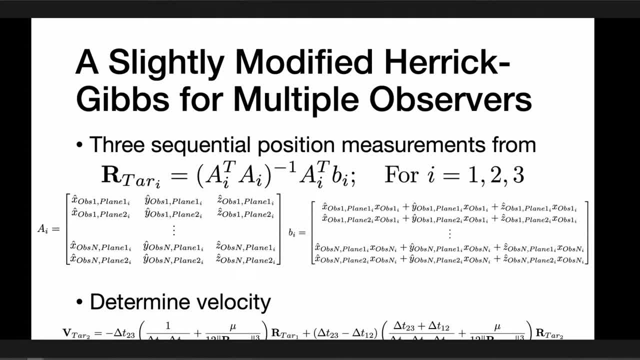 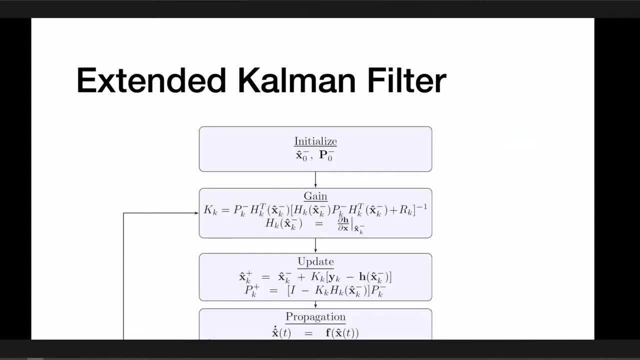 from n observers. essentially, In this case, we are representing a modification on a method called Harry Gibbs that takes three measurements and essentially estimates an initial position and velocity. This way, and as you can see here, there is some linearization going on in the filter, whether you are using the Jacobians. 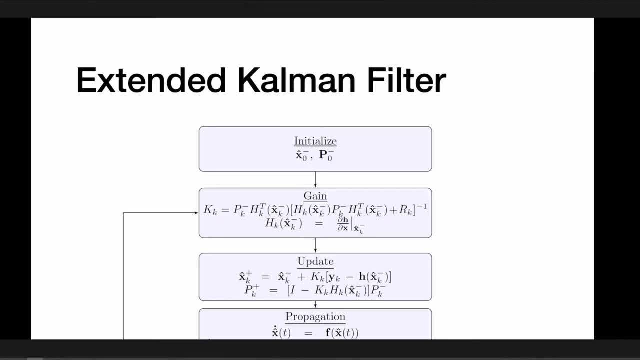 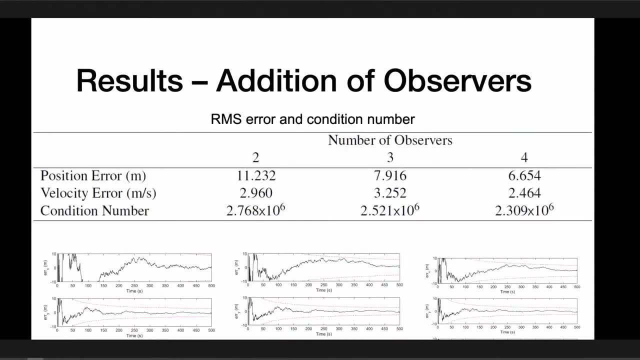 So this way you're close enough to a good initial guess and the filter would converge fast. Now we have done some studies about how, how, how, by how much results improve as you add or remove observers. So obviously, given the theory that we are basing it on, 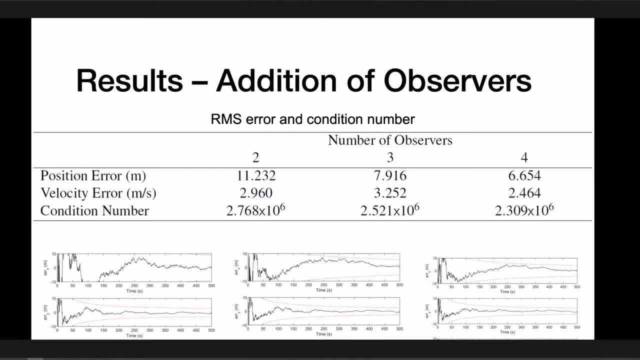 So obviously, given the theory that we are basing it on. So obviously, given the theory that we are basing it on, the minimum number of observers is two. Adding a third observer obviously buys some accuracy. Adding a fourth observer is not very obvious. 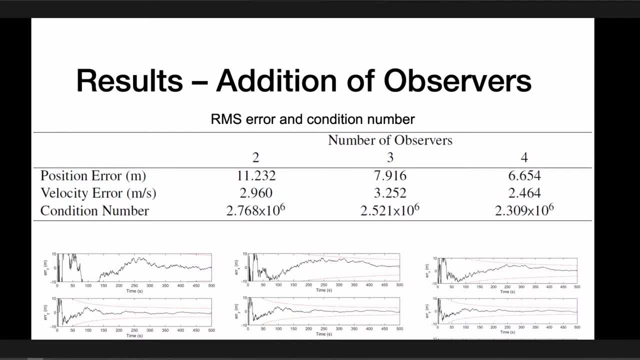 if you need a fourth observer, in terms of the RMSF and in terms of the overall filter behavior. So you can see there is a very similar behavior between three and four observers, albeit there is an improvement, but it is not that significant. So we did some studies to see how many observers we need and what is. 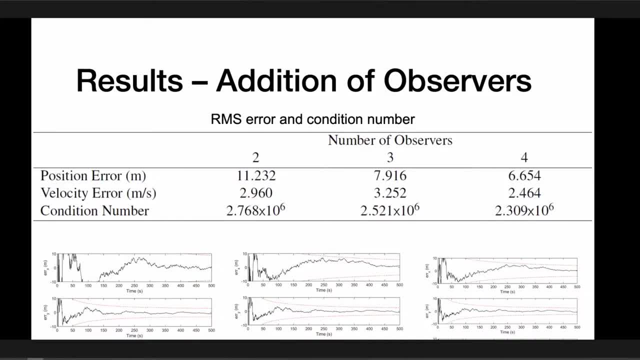 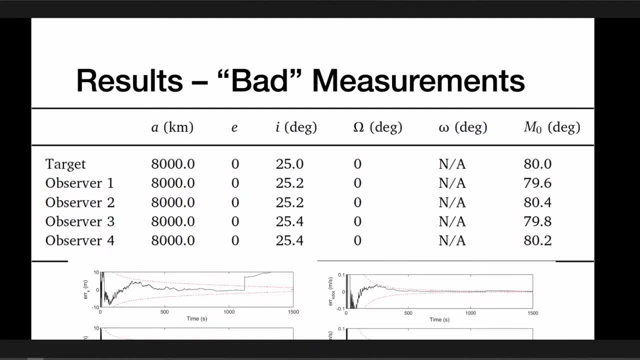 what would be an acceptable number of observers to obtain good results. The other effect or the other area, is that a filter: if you introduce bad measurements to the filter, the filter diverges, and that is universal. Any filter: if you introduce bad measurements, it diverges. 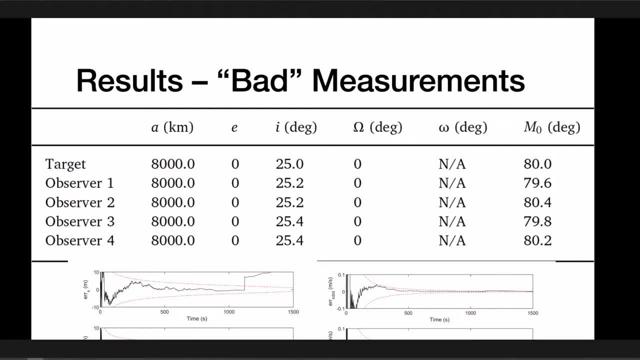 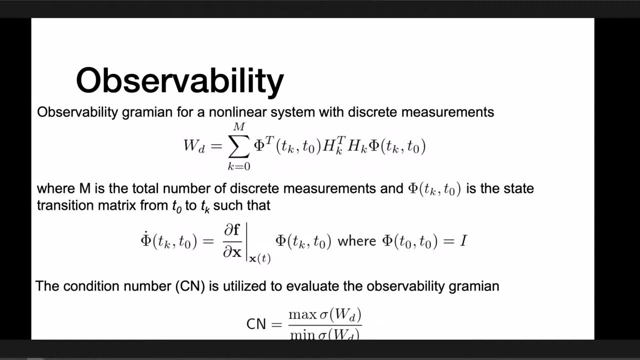 Now in our study is that we needed to define what are bad measurements in that context, What would entail a bad measurement, And for that we used this idea of observability. This set is, this set of results is based on an analysis that links observability or the instantaneous observability. 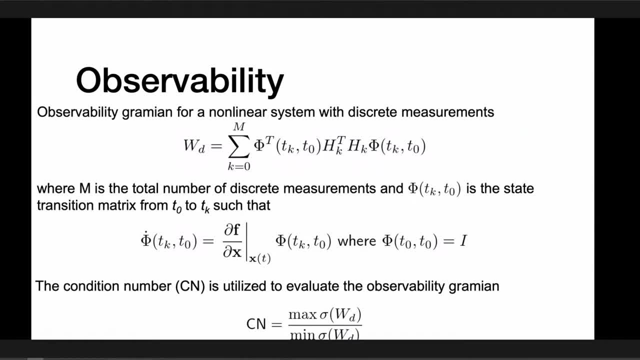 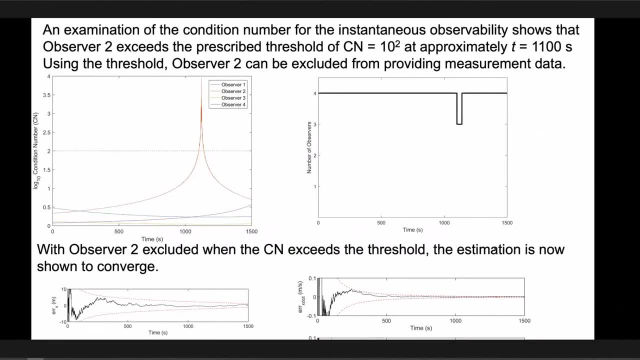 with a, with the accuracy or defines what is a good or a bad measurement. And for that we essentially came up with- sorry, I'm going to yeah- we essentially came up with a scheme where we can exclude a measurement. 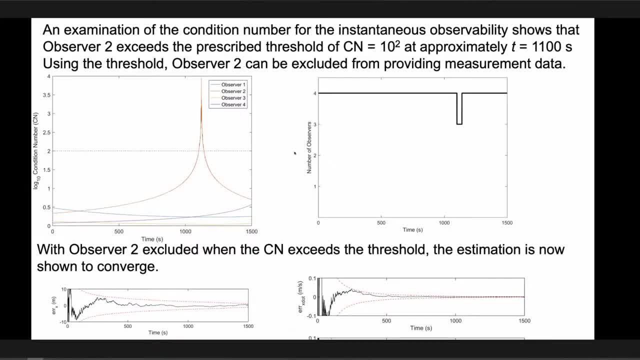 As you can see here, we came up with a threshold on the condition number for this specific research And essentially this: this threshold defines what a bad measurement is. So now you can see here. we start with four, two observers. When we reach the threshold, we turn off one of them. 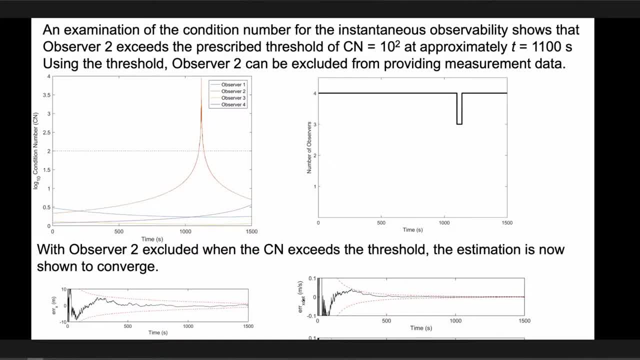 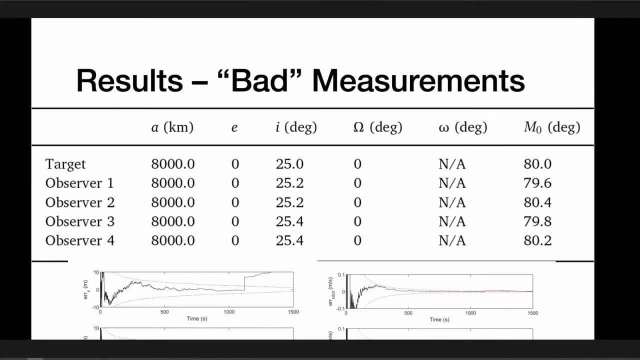 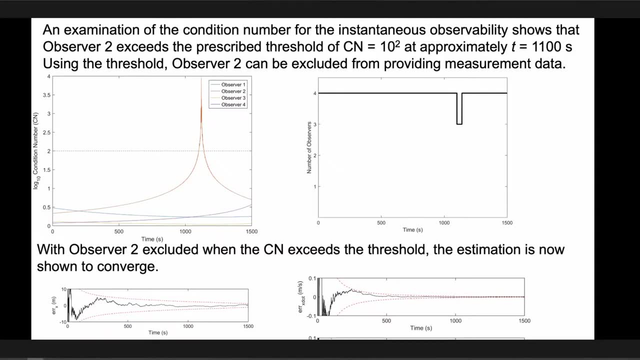 and then we turn it on again And you can see the effect of this, of this approach, on improving the filter results. So, as you can see here, the previous one, the filter diverges and here it's in a much better shape, essentially converges to the previous levels of accuracy. 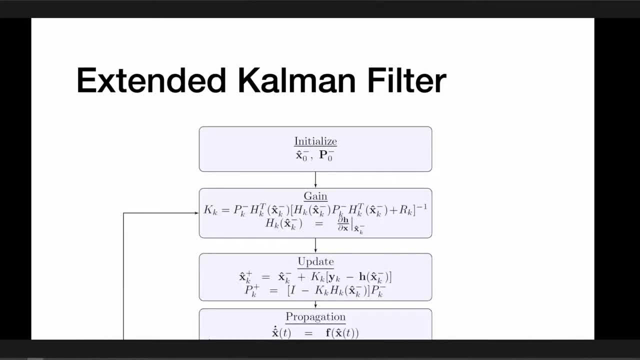 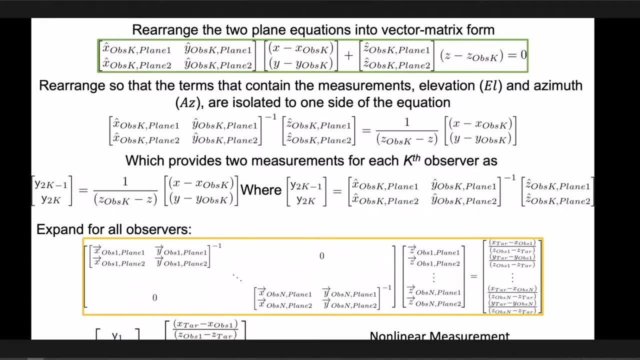 Which is something that is enabled by the fact or by the structure of this measurement model. As you can see here, all we need to do is just remove one of these sub-blocks and essentially keep going with our filtering scheme, right there. 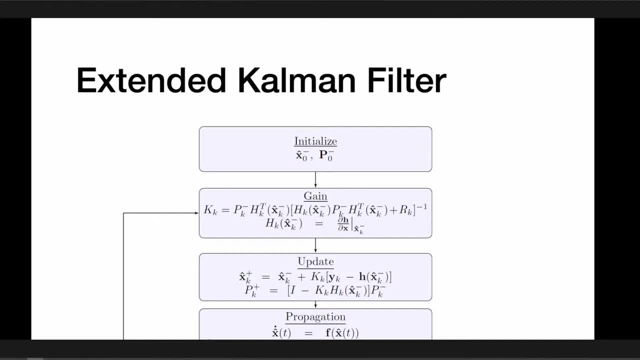 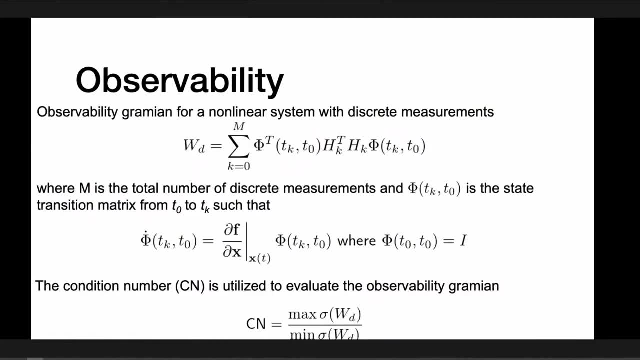 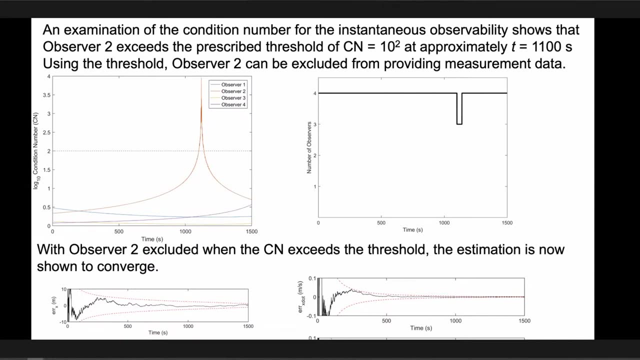 And when the fourth or the excluded observer becomes available back online, we add its sub-block and essentially improve the results. Now, this could also be said for tasking: I could essentially turn off one or two observers out of the four. let's assume that the four are all doing well and producing good results and do not have an observability issue. 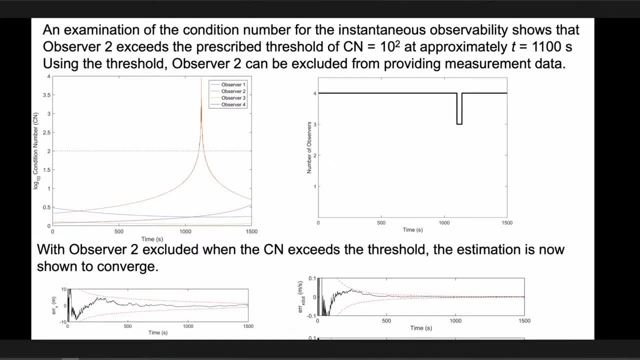 I could choose to select to turn off, to basically turn their attention to another object that they need to track. As long as I have two looking at an object, I still can get very good estimation results, So that versatility is enabled by the measurement model. 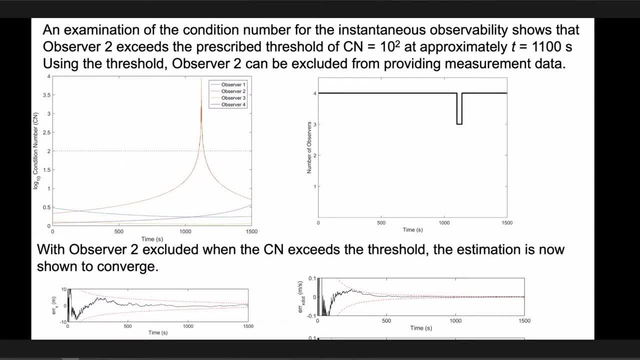 and essentially it can be turned on and off, depending on whether it's a bad input that will cause the filter to diverge, or tasking, Because later on what we found out- and I'm not showing those results here, but rather we can actually adapt the measurement model. 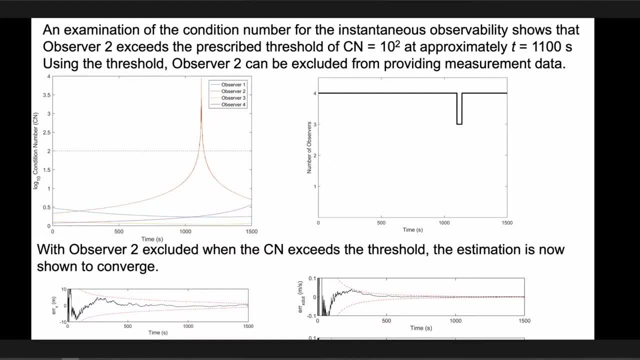 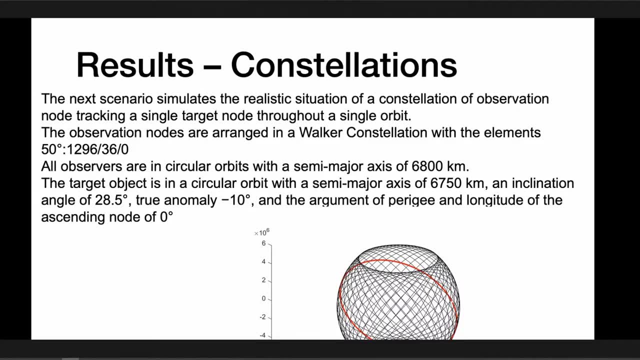 So we avoid this singularity or this jump in the condition number. So we moved on to applying this on a constellation, And this is not an optimized constellation. This is a standard Whopper constellation looking at the sky. A Whopper constellation is what you see here in these criss-crossing path of a couple of thousand satellites. 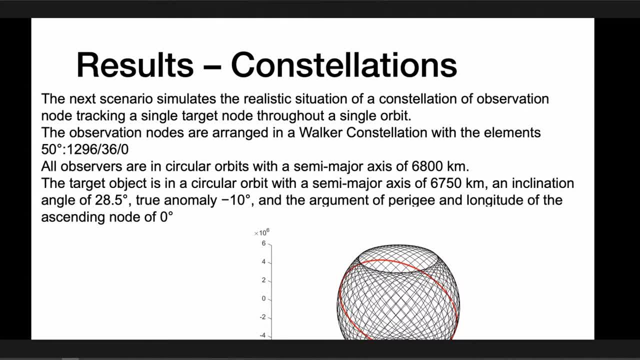 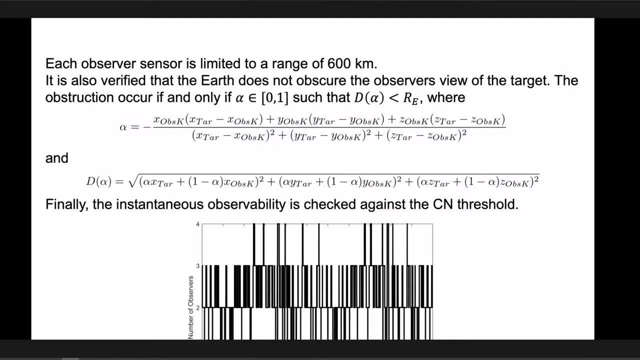 So this is not optimized at all. It is just a representation of a constellation that could use could be used to track debris in an Earth orbit, And you can see here now we included another factor, which is Earth obscuring the object. 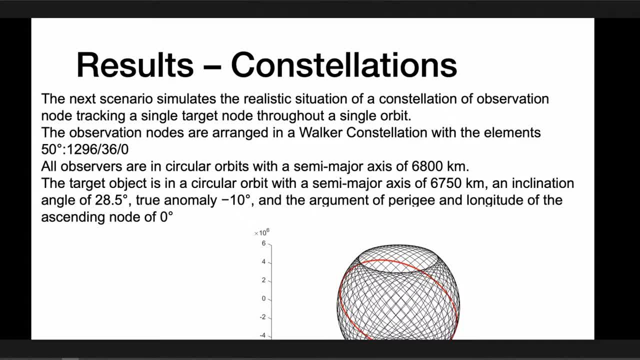 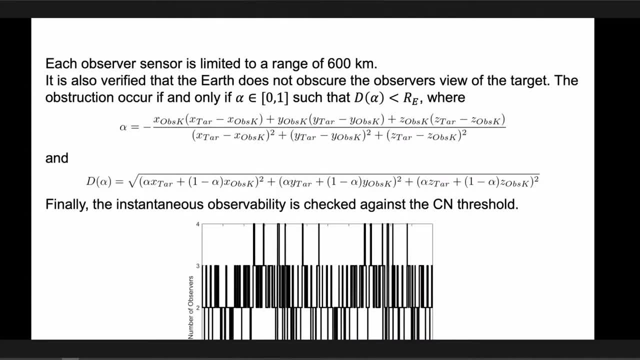 Because you see here, some of the path are on the other side of the planet, assuming that the planet is in the center of all of this. So if you look at this, this plot here shows how many observers are being utilized throughout the whole simulation time. 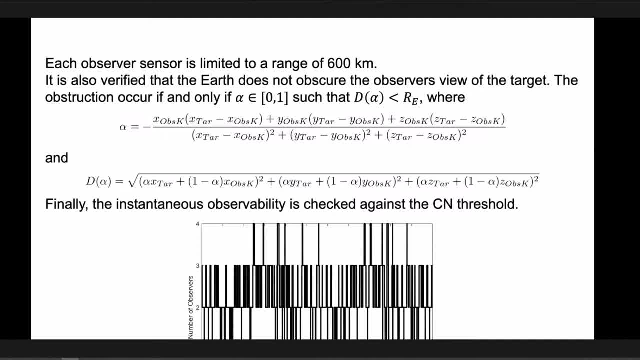 And there was a limitation on the range. There was also a limitation on Earth being in the way, And we can also add several other limitations And also we could also add tasking. In addition, we in this simulation, we also had the condition number threshold. 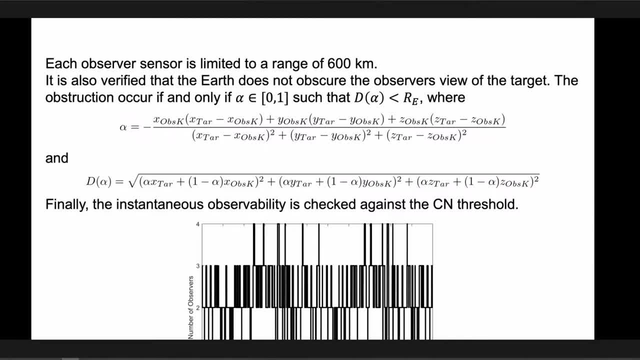 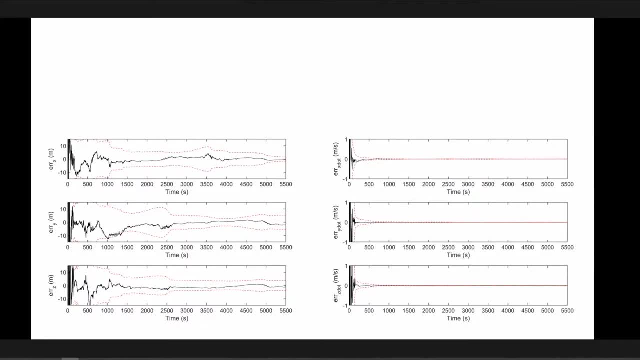 So here we only considered three factors: range, Earth and the condition number, which essentially exclude bad measurements. And you can see here how the filter behaves or how we can include and exclude measurements In our observers as we go forward And the results are, as you can see here are, very good. 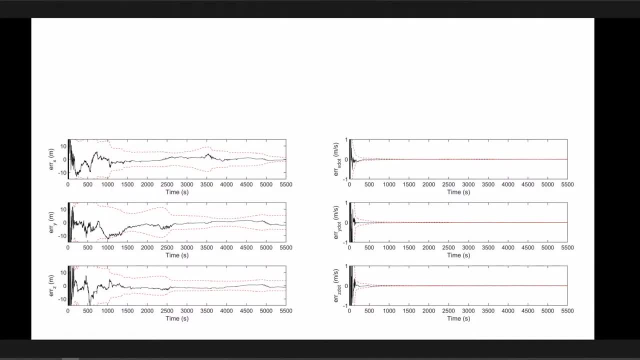 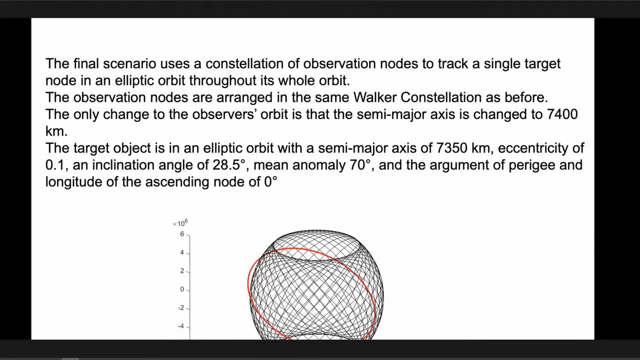 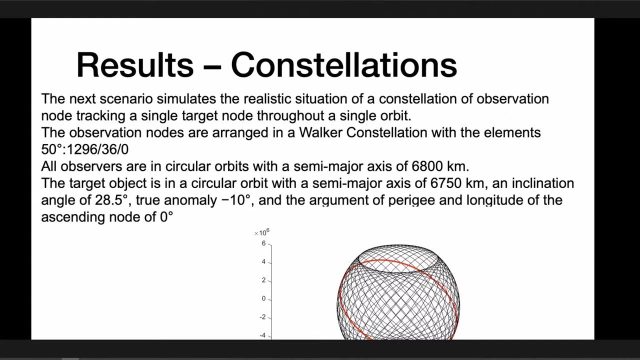 We talk about meter accuracy of position and velocity and a good sensitivity result. Then we move to: so here the assumption here, although it might not be, might not be showing because of the scaling of the plot, but this is circular orbit. 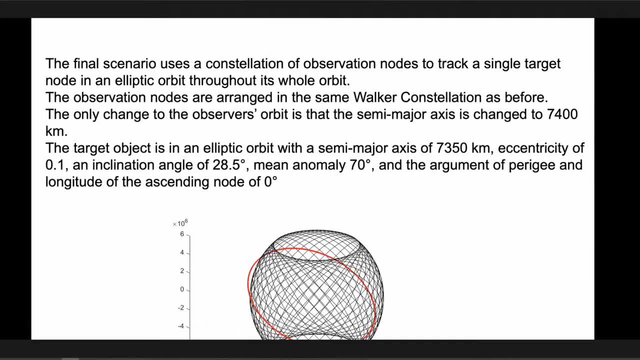 The target has a circular orbit in in astrodynamics, As you increase the eccentricity of the orbit, you increase the difficulty of the problem, You increase the non-linearity of the problem. So here we introduce a slightly eccentric orbit, a 0.1 eccentric orbit. 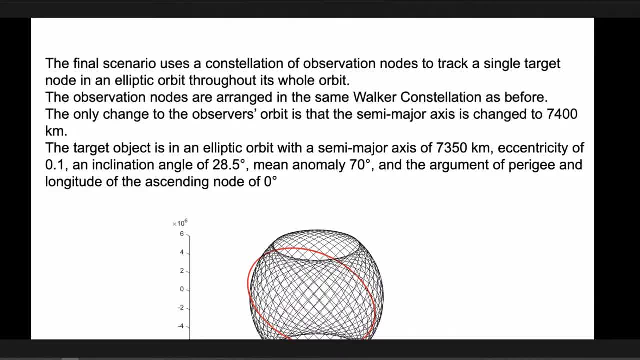 which is not a small eccentricity. Most of Earth's orbiting satellites in LEO has a lower value than this, but still not a very high eccentricity as well. So we introduce the 0.1 eccentric orbit And again you could see here that because of the eccentricity, 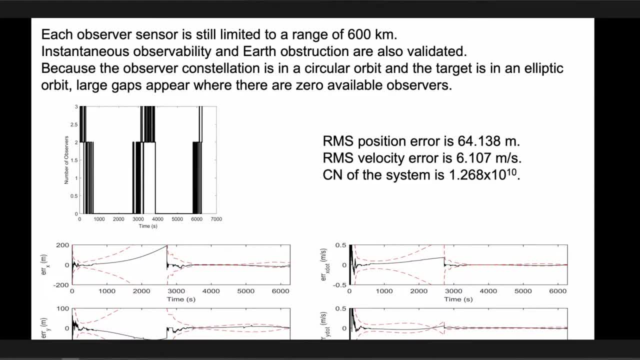 and the various constraints we put on the filter, the number of observers that are being utilized has dramatically decreased. However, we're still within the same order of magnitude of estimating both position and velocity, And you can see that the filter behavior here, especially in these increasing gaps of 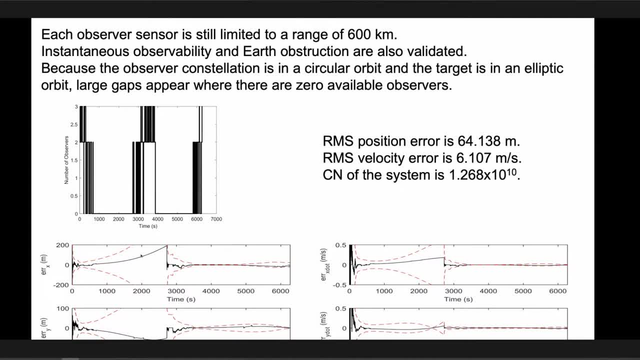 no measurements. So you can see here that the bounds or these red lines describe the uncertainty bounds of that filter, that the filter is getting or moving towards diversions. But once we start picking measurements again, it quickly converges and finally converges to the final. 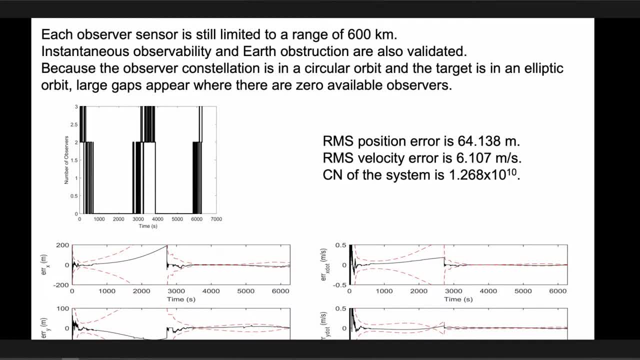 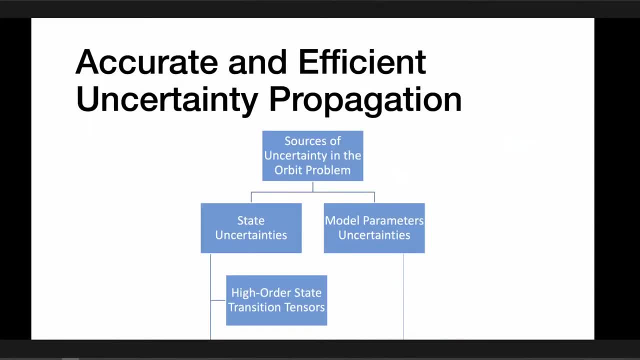 to the accurate state estimation. So that also is a function of the robustness of the proposed or the shown measurement model. So as you see here, the filtering problem has uncertainty embedded in it. So this is basically that the second part of this astrodynamics research is that 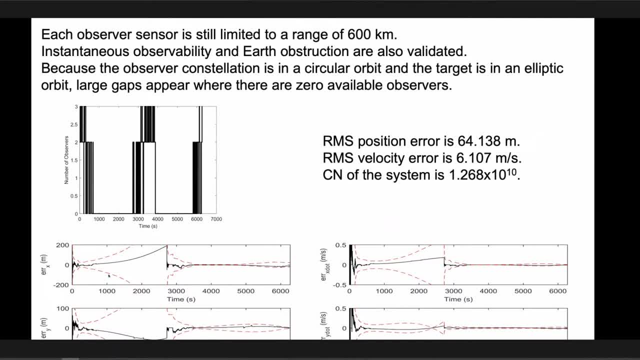 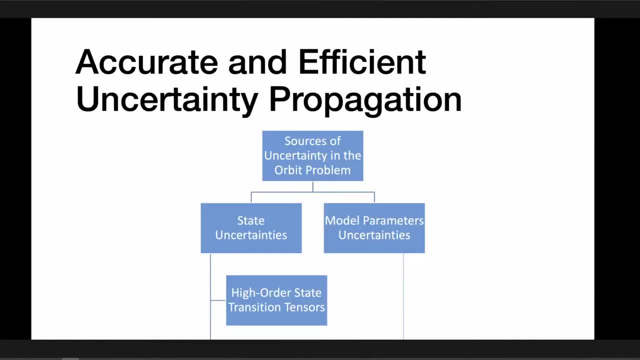 as you increase. as you see here, these uncertainty bounds are also an intricate part of the estimation process And that gives me the confidence levels of my estimates. So sources of uncertainty in the orbit problem in general can be divided into a couple of things. 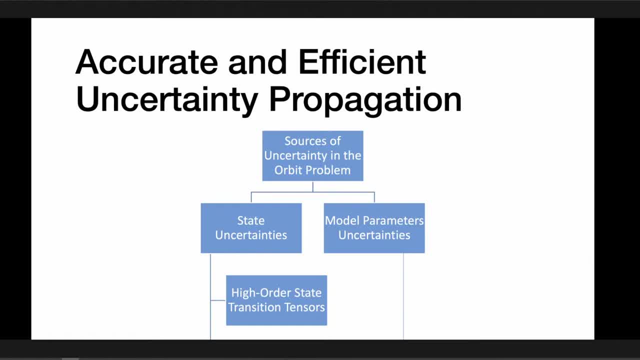 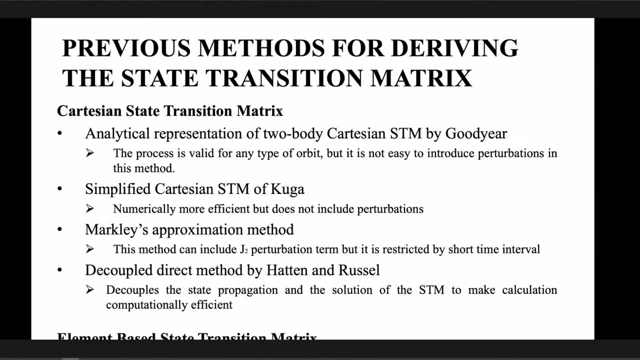 It could be divided into the statement, the state uncertainties, and this is how the uncertainty surrounding my, my best guess on the current state position and velocity in inertial space of a target or of an object in space that I am tracking And, essentially, in the filter. this is what this is. 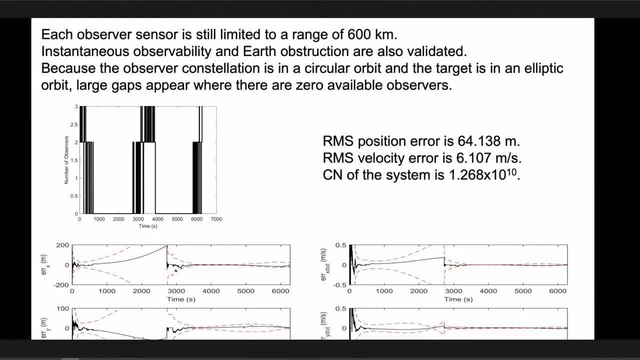 This is the red dotted line that essentially described the three sigma bounds of the three sigma uncertainty bounds of of that. So, as you see, as the filter is converging, also the uncertainty is converging, which means that I'm getting more and more confident in my estimate. 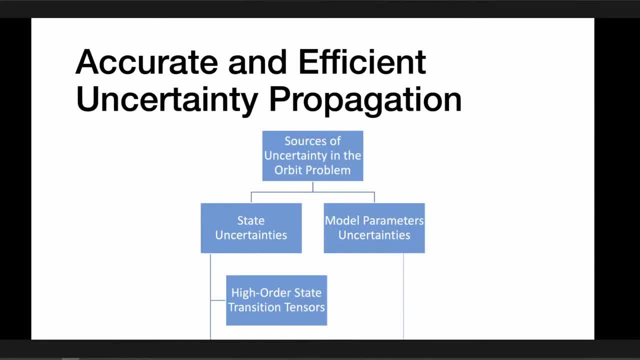 And that's a very important factor. The other area is that there are parameters in the model, not just the, the state uncertainty. The model has constants, or what we assume are constants, that are related to the gravity model, the drag model, the solar radiation pressure. 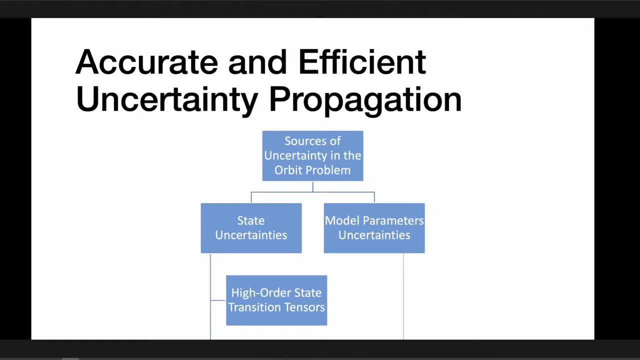 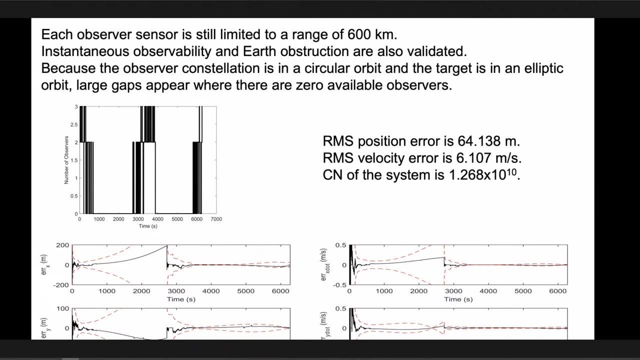 all perturbations that go into the model And those uncertainties also are introduced in our propagation. The other thing is that motivates this uncertainty of propagation business is that when you look at this plot very specifically, you will realize that for space-based surveillance, 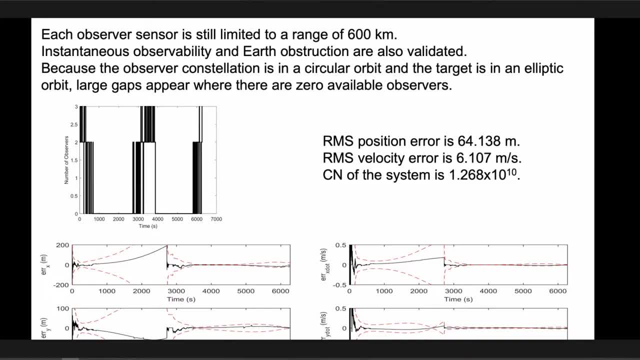 there will be gaps in coverage, and significant ones, because of range, because of lighting, because of because of tasking too. Now, this problem can be resolved by constellation, design, optimization and so on, which is something that we are looking into, But assuming that 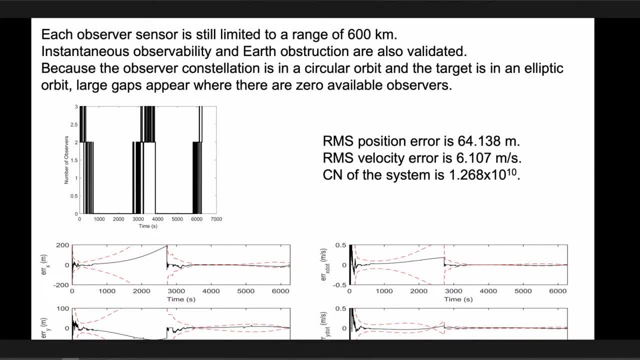 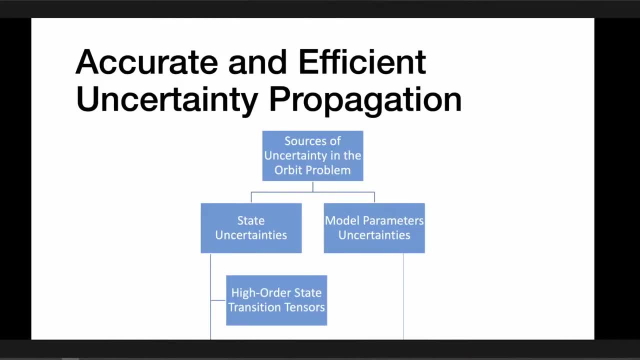 you know, even with all of this, there will still be gaps, And as the gaps increase, you could see that your filter diverge. And that is essentially what motivates looking into these uncertainty propagation Two approaches that we are looking at. is that essentially how to? 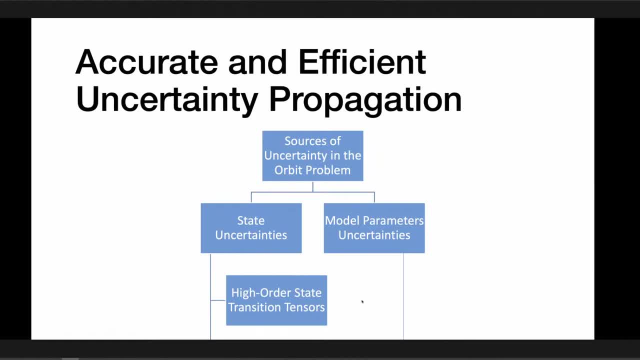 compute the state transition tensors- high order state transition tensors- and how to approximate the probability density function, And both of them have uses in collision, in estimation, in prediction and and in general. all of that obviously feeds into having better space situational awareness or more robust space situational awareness. 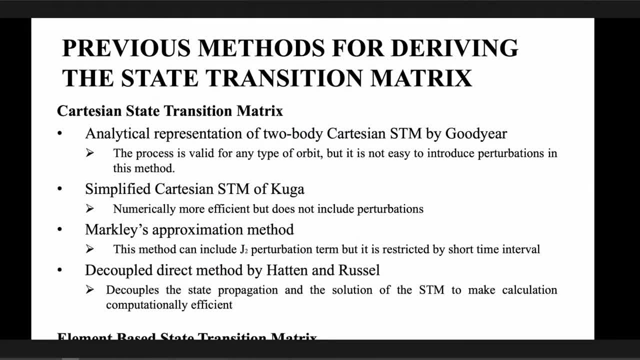 So we'll start by looking at the state transition matrix. Several works have been done looking at Cartesian space state transition matrix, some computation techniques to compute the STM with and without perturbations and also some that have moved the coordinate frame from the Cartesian coordinate frame that we have been looking into. 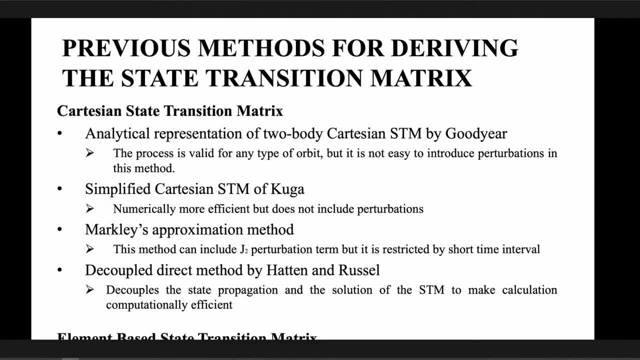 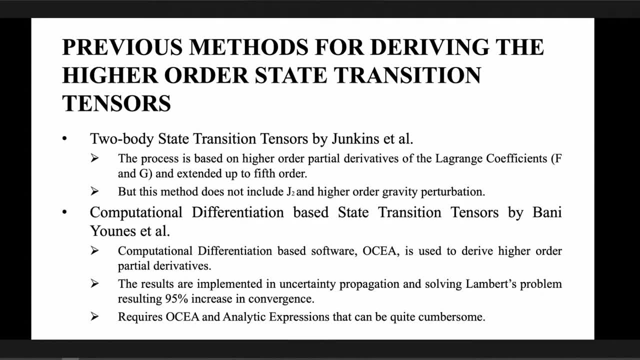 to an element based coordinate frame which refers, which can essentially produce a different set of results or more amenable results. What we have looked at is is what we looked at is essentially using a method that is along the lines of automatic or computational differentiation. 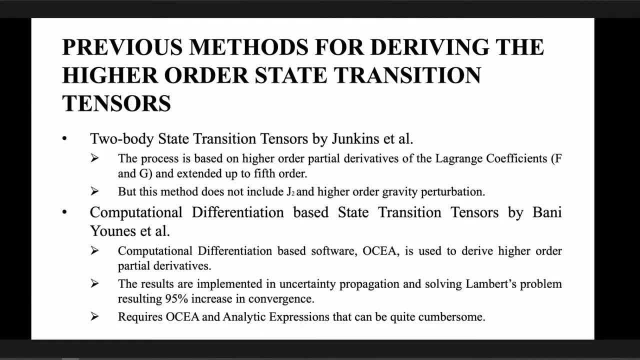 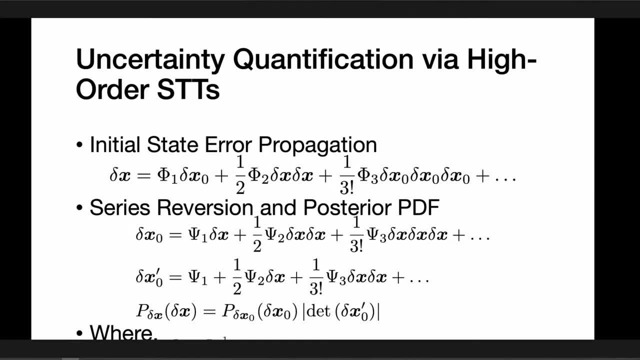 that can essentially compute those values using some recursion functions, And I'm going to show this next, but this is what it could be used for. So if we look at the state transition matrix- and usually we represent this in astral by phi- 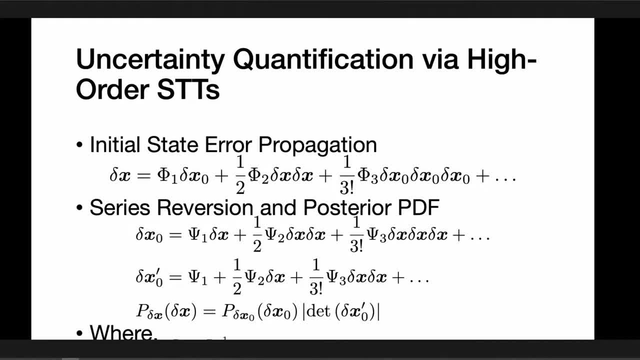 these are the higher orders ones. So this is the first order. This is an n by n matrix. This becomes a tensor which is an n by n by n tensor. and this is becomes a fourth order tensor which is an n by n by n. 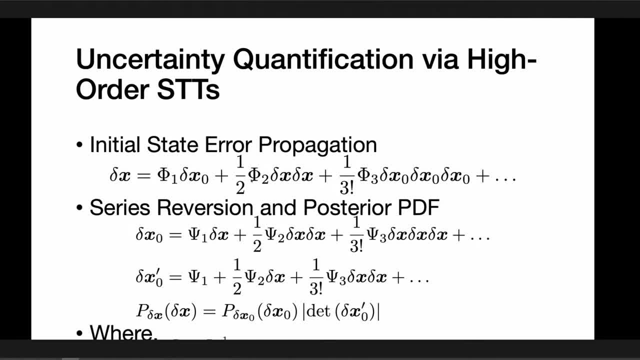 and so on. So you can see here, this is six by six, six by six by six and the orbit problem. this orbit problem has six values and this becomes six by six by six, three of them, and so on. 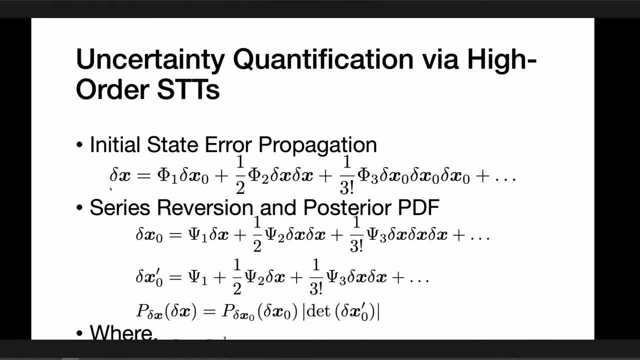 So essentially this is the variation, and the variation in the final state is a function of the variations of the initial state right there, And you could essentially come up with the distribution function of the final state, given the initial state, through that sort of reversion of the series. 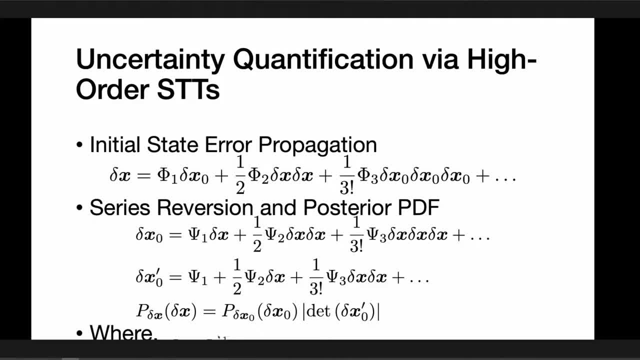 And these are the coefficients that you come up, come up with Now. the inverse of phi is: is can be easily computed because phi has a something called it's symplectic. So, because phi is symplectic- and we'll discuss this later- 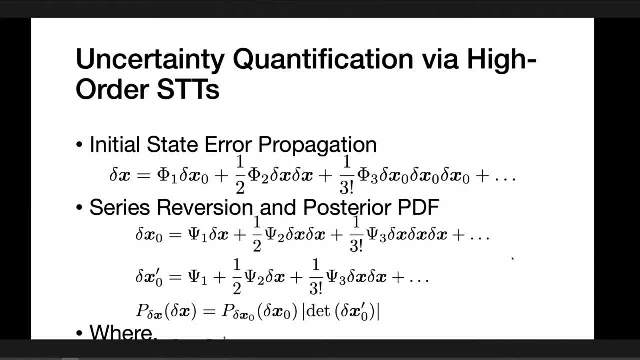 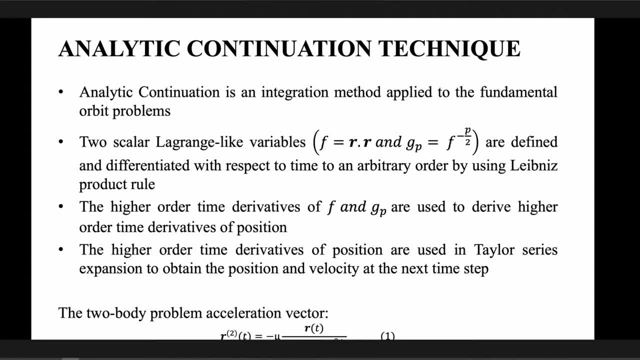 its inverse is is is not as complex as it would look like, But what we are, what we have been exploring, is a recursion, recursive technique that essentially represent the two-body problem in terms of these scalars right there: an F and G scalar. 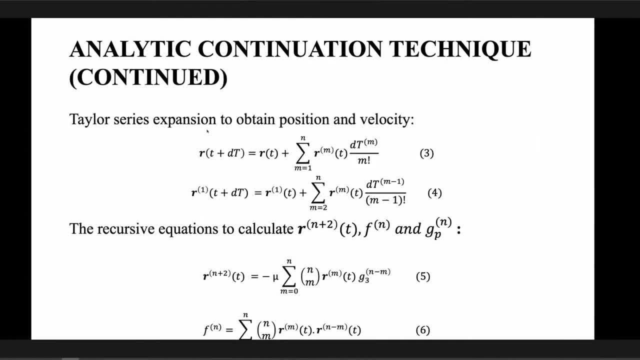 And we used what is essentially the chain rule or, more generally, the Leibniz rule, to come up with the recursions for these values. Now, if you look at this, I can essentially tailor, expand the solution of the position and velocity. 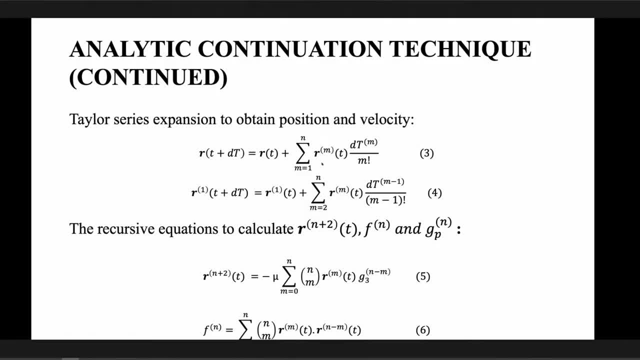 but then becomes a function of the higher order, actually, like the higher order time derivatives of position, velocity, acceleration, jerk and so on and so forth. And if I can compute those guys then I can essentially sub in the Taylor series. 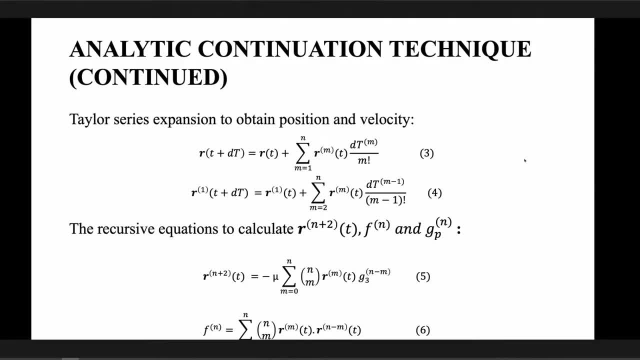 and I can go to any order. Now there is, there is- and we've published a few papers about this, essentially showing that this can go to up to 25 or 26 order, make bigger jumps in the time, And we even came up with some optimizations to find the best time and the best order combination for an accurate solution. 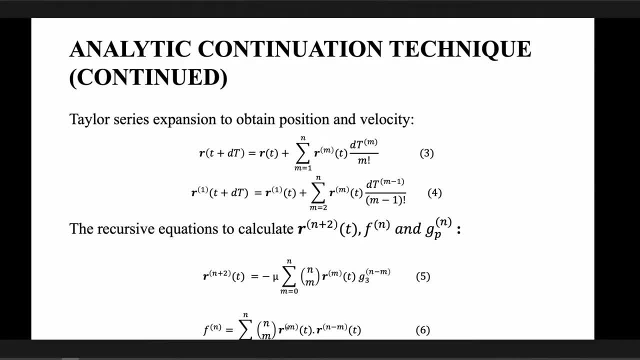 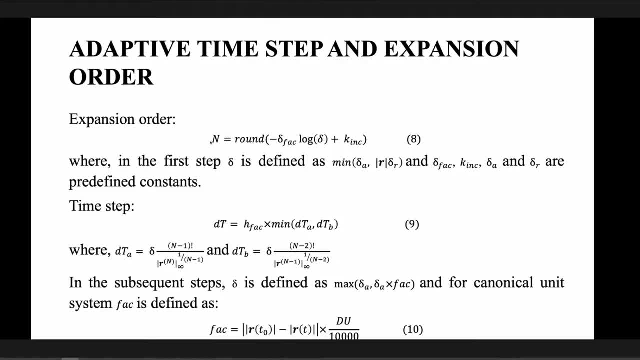 So that was all well and good and we were able to produce those recursions- And this is what I was just describing about the adaptation of the method- that it essentially come up with the best n, which is the number of terms in that Taylor series, and comes up with the best delta t. 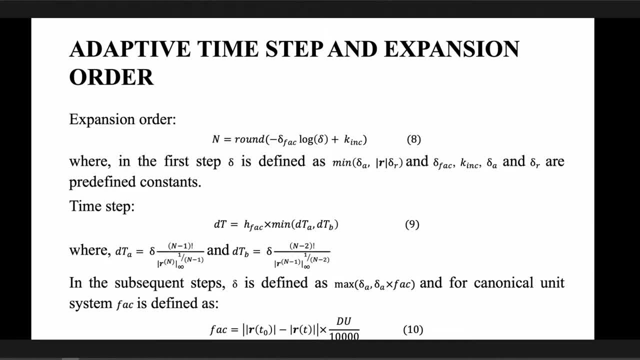 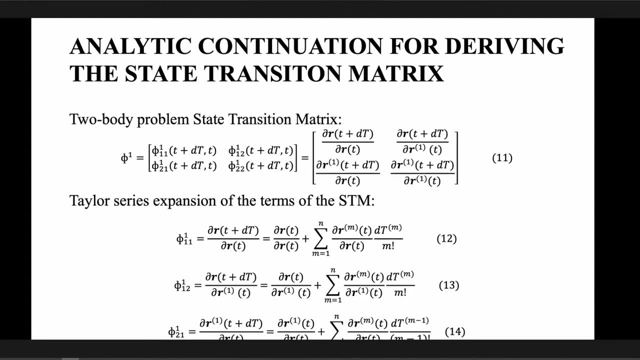 which is the distance between each point that we are evaluating that. So that's based on the last two terms of the series, and, and a prescribed relative and absolute tolerances. But this is what we were looking at when we looked at the state transition matrix. 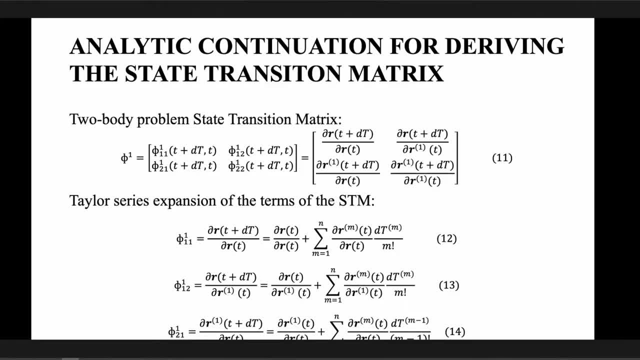 is that we can use the same approach to come up with the various elements of the state of the state transition matrix. So the first order state transition matrix right there which is has has that superscript one- is a six by six matrix that measures the sensitivity of the position to the 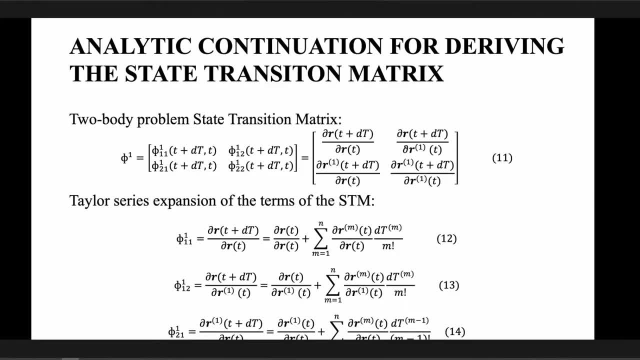 the initial position, or in this case, just the previous position- and to velocity and then measure the sensitivity to pull velocity to position and velocity. So if you use the same approach and you expanded the Taylor series, you will get these expansions Now. 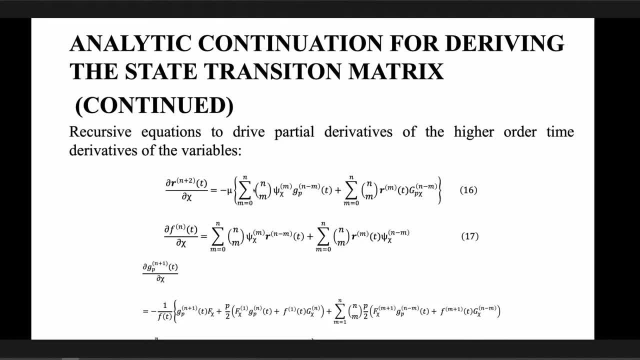 we followed the same idea of essentially coming up with the recursions that describe these partials. So you can see, here there is that application of line net product rule for the partial derivatives or the higher order time derivatives of the partial derivatives. 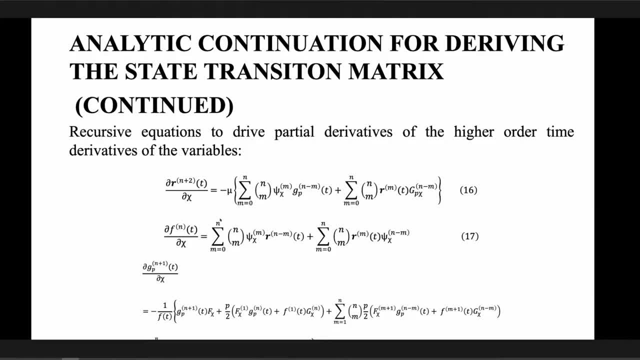 If you see equation 16 and 17, and we came up with those variables. Now, as you go higher in the dimensionality and you can see that the only term there is- there is only one term- that gets added every time you go up in a dimensionality. 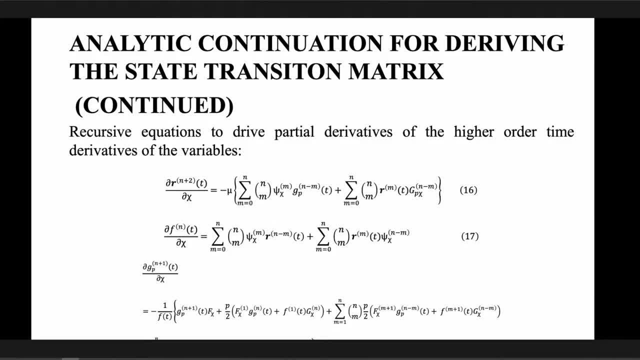 And this term. once you know the first value of it, you can essentially keep recomputing the higher order derivatives of it recursively. So with that in mind, we essentially can reproduce what we did in the state, in the state variables to produce the state transition matrix. 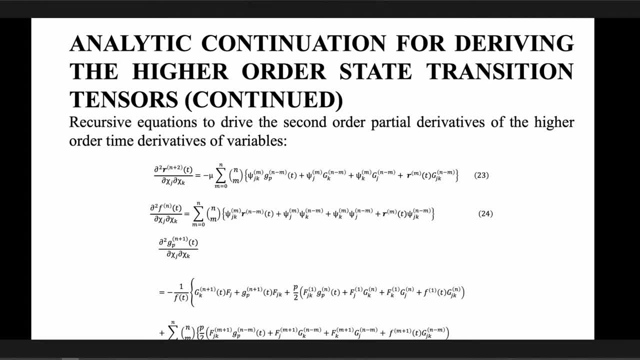 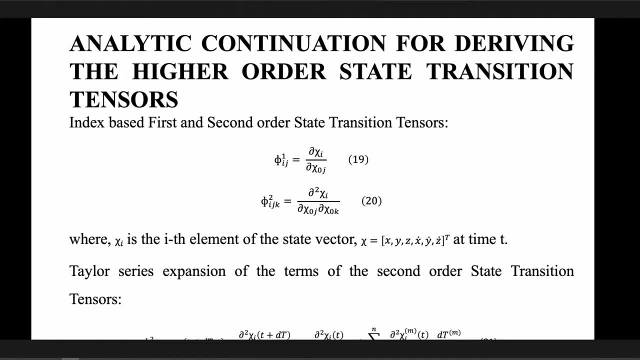 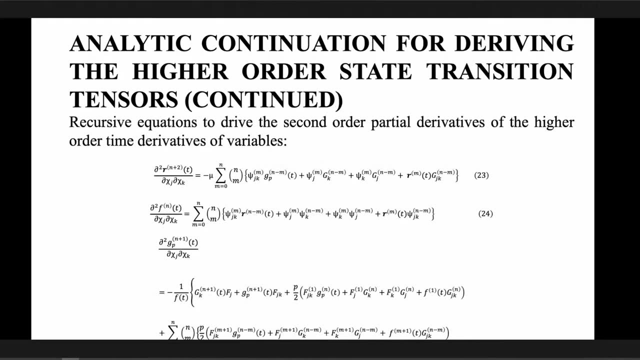 which essentially what we have done here for the first order, as you see in the previous slide. Now the second order, you see, now we're using that index notation where we have the second partials With J and K, And that what this recursion look like. 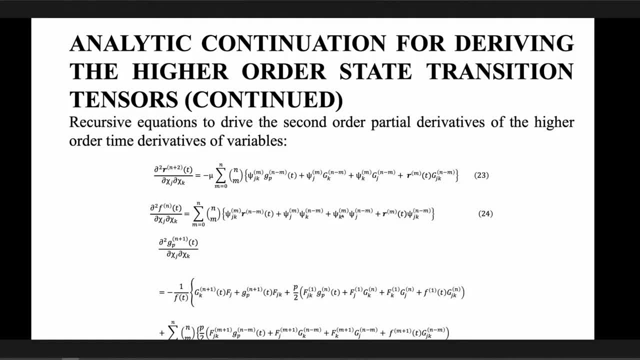 Now again, you can see here that from the previous term there is an additional two terms. but that but those, all of them can be computed recursively, So we only need to evaluate the first one Anytime you introduce a term, you just need the first value of it. 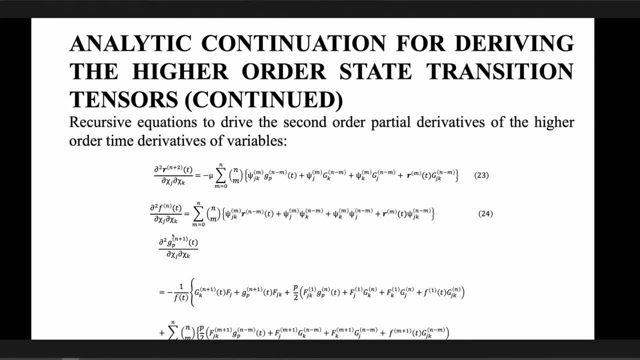 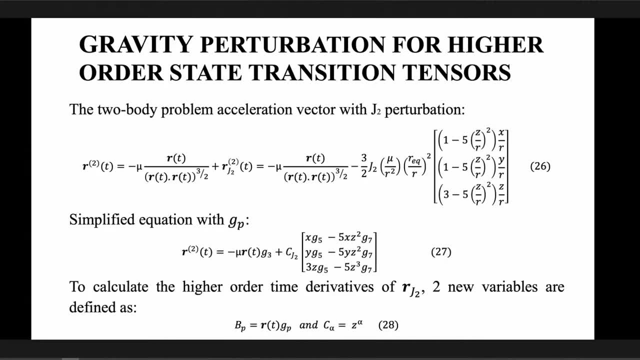 And then the higher values comes from the recursions. Uh, as you see here in R and F and G and so on. So we added some perturbations to the model and perturbations are important. The G2O perturbation is one of the most dominant perturbations in. 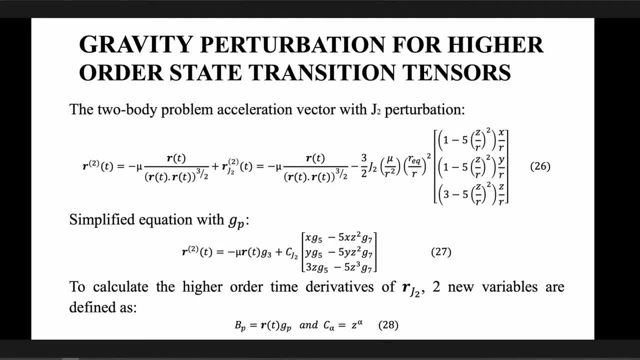 in the higher orders matrix, in the in in in astrodynamics, And it accounts for the obliqueness of the earth, essentially that the earth is not, as a perfect sphere. And uh, basically, we did follow the same approach, using Leibniz product rule and computed the 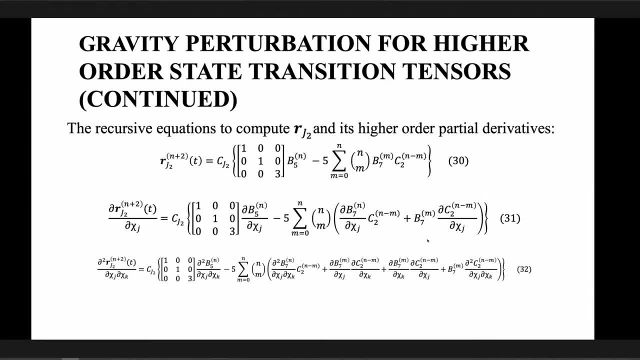 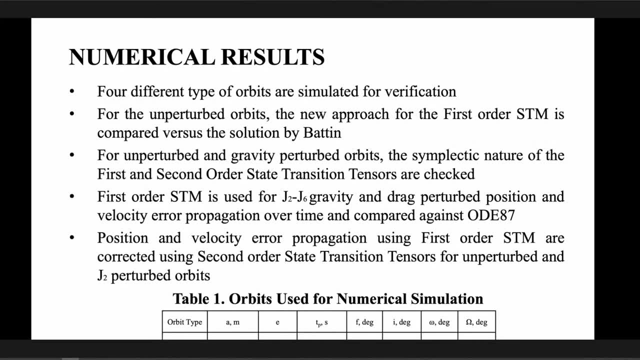 recursions in, in, in that perturbation. And that are, those are the set of equations that describes those recursions. We also have several results that show drag, that show a high order, uh, uh uh. zone of perturbations. 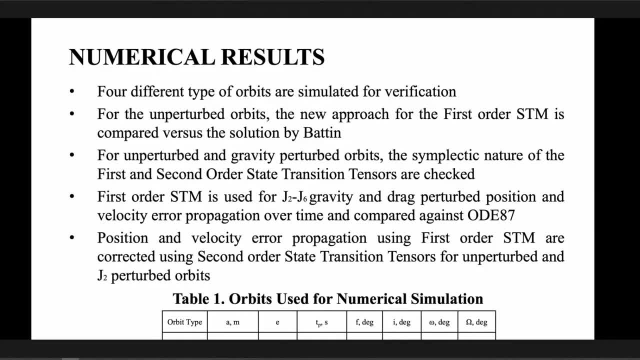 J2, J6. And we are also now working on more uh results related to uh, the uh, the more general perturbation model. So we tested this idea on several orbits and you see here the increase of 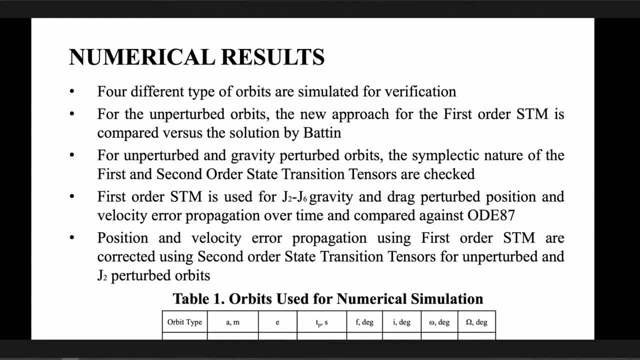 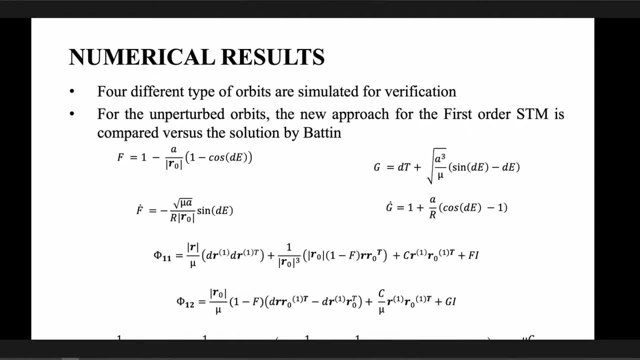 uh, eccentricity means an increase of the non-linearity of the problem and, obviously, the complexity of the computation. Uh, I'm going to skip this because we compared the um. so, without perturbations, there is a closed form solution that we compared against. 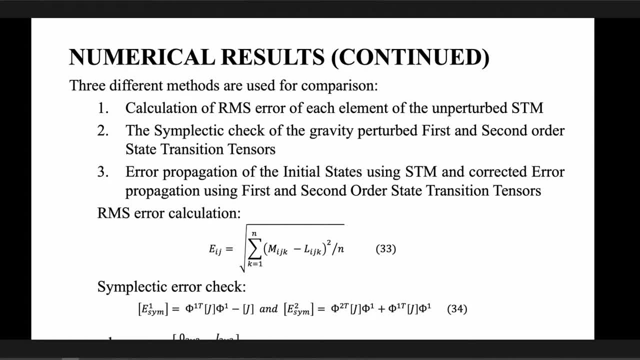 And this is the approach we have used to essentially come up with a way to validate this method. So we did an RMS error, We did the symplectic check, And this is what I mean by the symplectic property of that matrix is that the first order matrix multiplied by this skew, symmetric matrix. 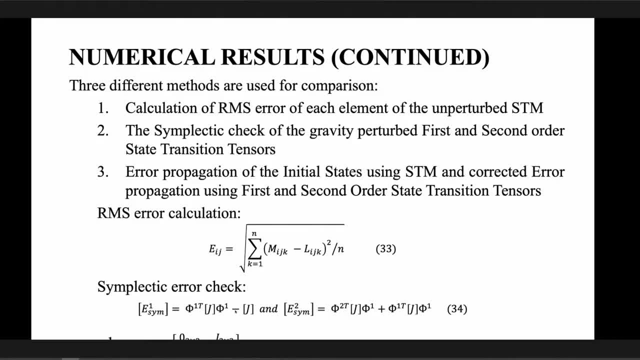 of the identity matrix, multiplied by phi again, is equal to J, which is this. So if you want to invert this, you essentially get the inverse of phi is it becomes J into phi, into phi, transpose again. So it's. this is why the inverse of this guy is very simple. 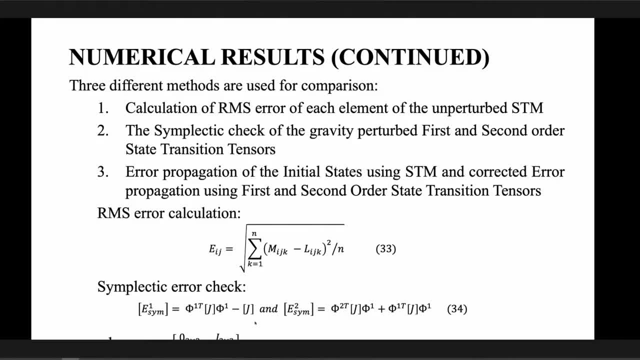 Uh and uh yeah, so that's uh. that is uh what we have, And essentially the higher order symplectic check is that you essentially take uh, the, the derivative, and that becomes uh, the check that we are looking for, that those two have. 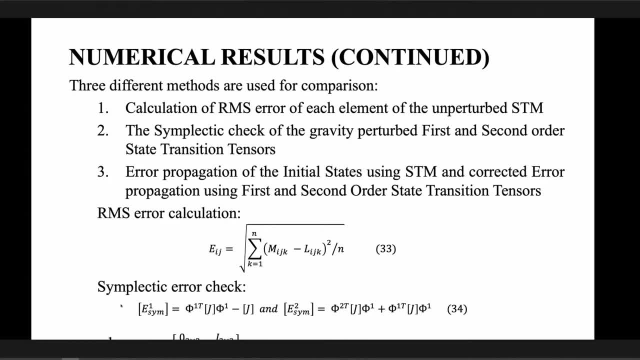 uh, uh, uh uh uh are equal to zero. So, with that being said, we can do this symplectic checks on the perturbed case without drag, because drag is an unconservative force And symplecticity is obviously connected to Hamiltonian or conservative systems. 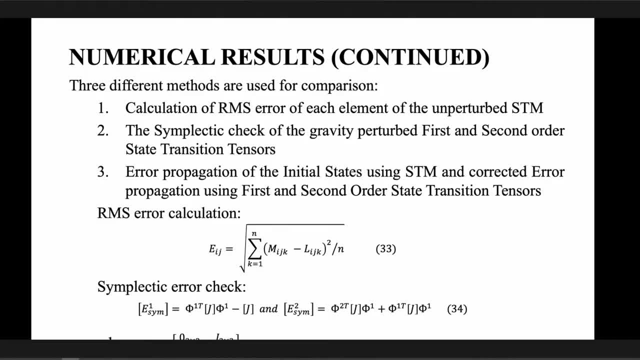 And uh also, the other way is, when you have an unconservative force, you use error propagation. So you estimate the error via the first order and estimate the error via the second order And you can see this comes back to the quantification of the uncertainty. because once you can estimate the error, 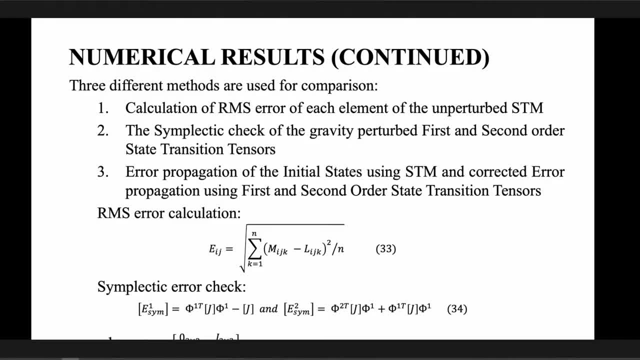 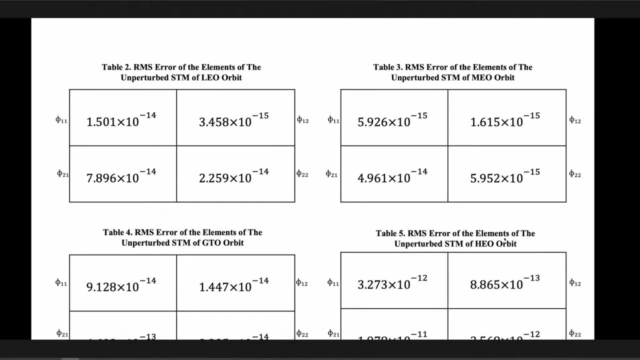 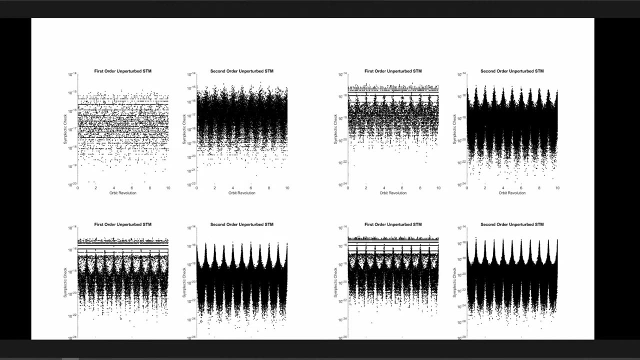 you have an idea about the variation of that variable And now you can put the uncertainty bounds related to that variation. All right, So we did several checks here. for the first order, the second order, double precision, and we are talking 10 orbit revolutions across the board for the checks that we did for all the orbits. 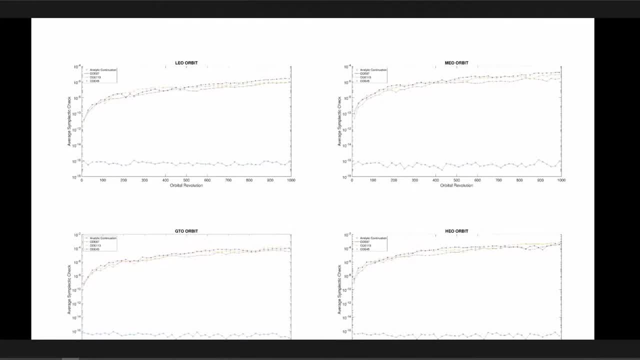 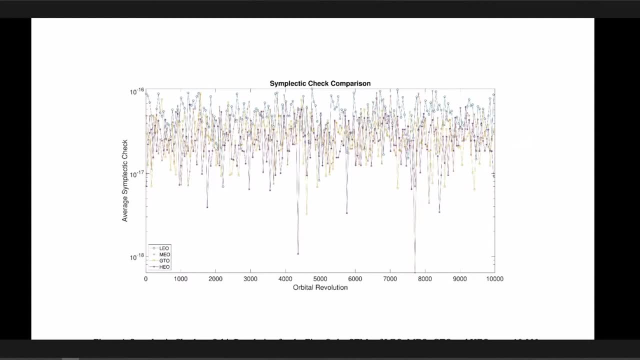 So, Leo, MEO, GTO and highly eccentric orbits, And uh for, uh for, to check the accuracy of the method numerically, we even pushed to 10,000 orbit, which is not realistic, And you should not do this for the state transition matrix. 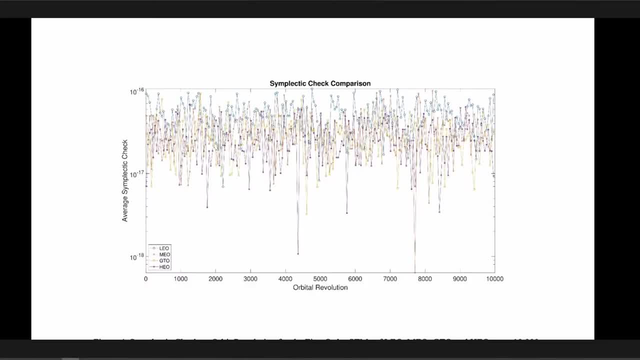 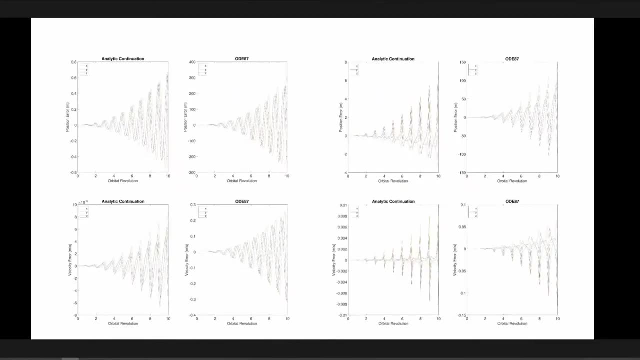 but this is just to show that it keeps the simplicity, uh of the state transition matrix up to 10,000 orbits. That check is mainly for the numerical accuracy of the of the method and not really for any application, as we're going to see later on. 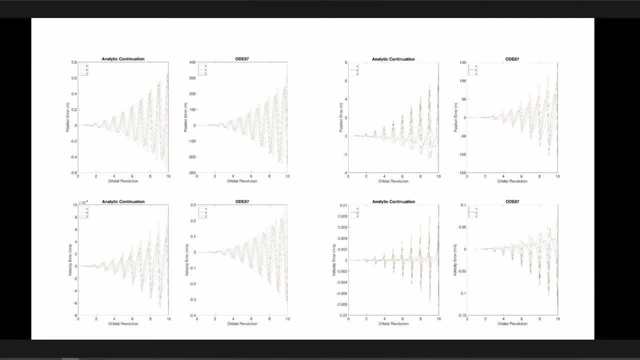 So here, when we introduce drag, you can see that as you increase the number of orbits, your, your values or your estimates or your errors are diverging. They are increasing with all. Now we are talking here 10 orbits, which is a very significant. 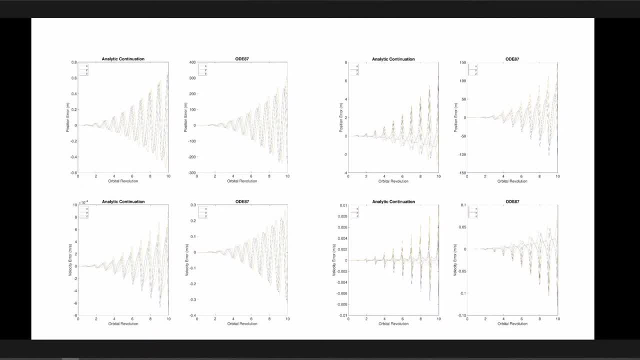 uh, extent of, of the, of the error prediction, And you can see here there's a couple of orders of magnitude between position and velocity estimates throughout the results, across all results. But as you also can imagine that even though the state transition matrix is symplectic, 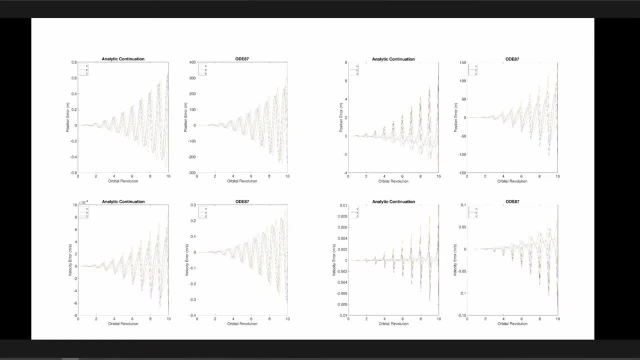 or, as you can also see, even though the state transition matrix is symplectic up to 16 digits, which is the extent of double precision, we still are using digits. We are in the second or the third digits in in meters and meters per second. 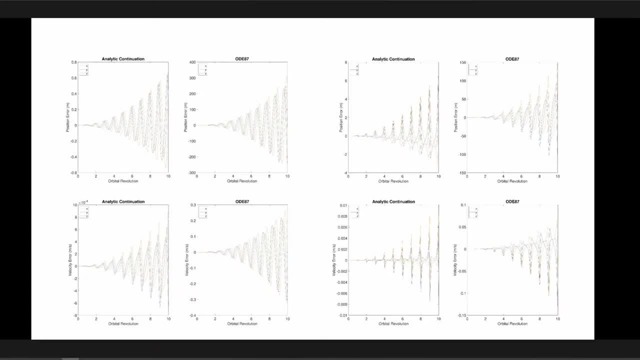 in terms of uh, in terms of orbit prediction, And that's why, for 10,000 orbits, you can see where this is headed. This is not going anywhere. uh, uh, anywhere, uh. we are in, in. 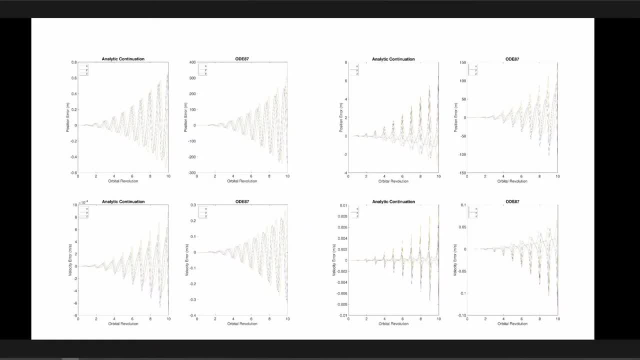 in in anywhere that is reasonably uh, representing the physics. But again it shows that the, in this case, the error is not coming from the fact that the state transition matrix is not accurate. This is coming from the conversions of the Taylor series. 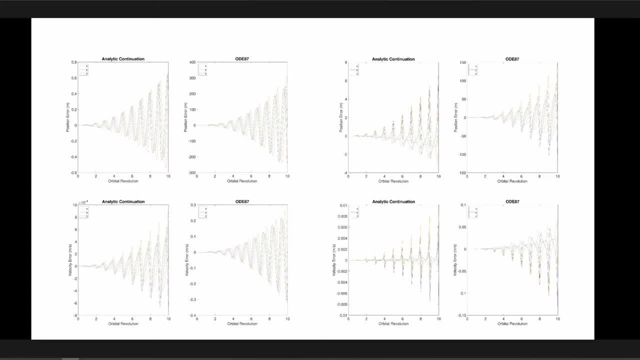 It's a. it has a radius of convergence And as you extend that measurement, as you extend that period of time, you're accumulating truncation and round-off errors And those errors cause the- and this is a property of any uh. 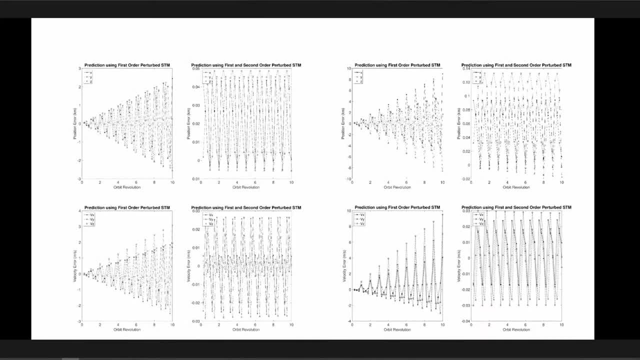 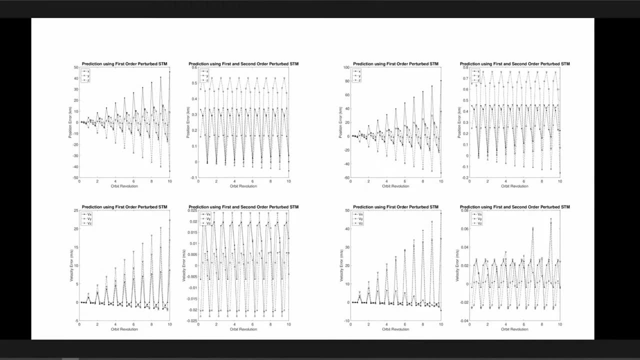 of any numerical method, So I'm going to skip this. This is just to show various orbits with various first and second order. uh, uh, approximation, Uh, but across the board you see the effect between. are we showing here the effect or the advantage of? 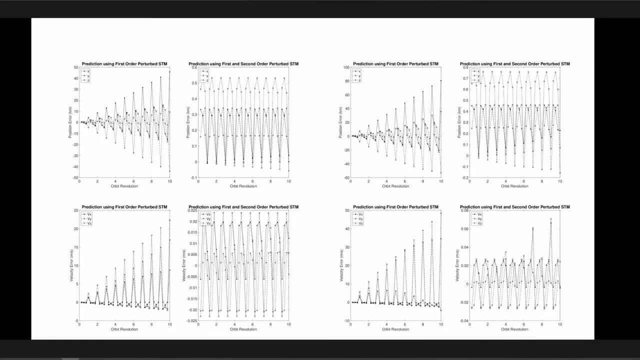 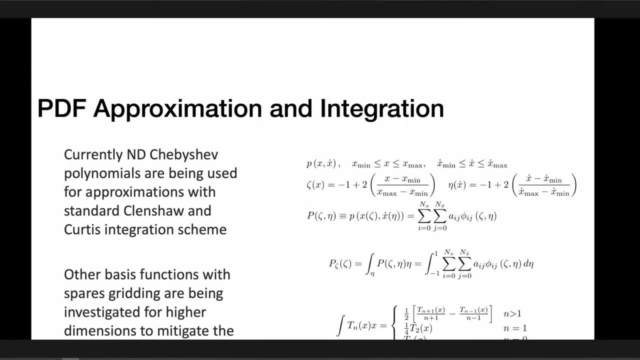 of getting an extra one or two orders of magnitude accuracy when you increase the dimension and you increase the the, the degree of the approximation. And we're now looking at the arbitrary order problem as well. Now the other aspect. that is okay. 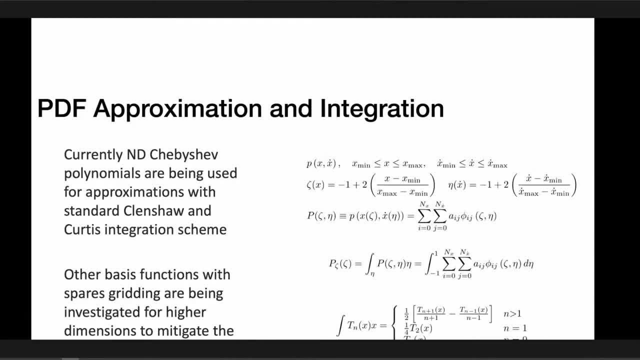 now we have this, all of this state transition matrix stuff which goes very well with estimation. As we have seen, there is a covariance matrix and this covariance matrix can be computed from the state transition matrix. But also there is- there could be- parametric uncertainty. 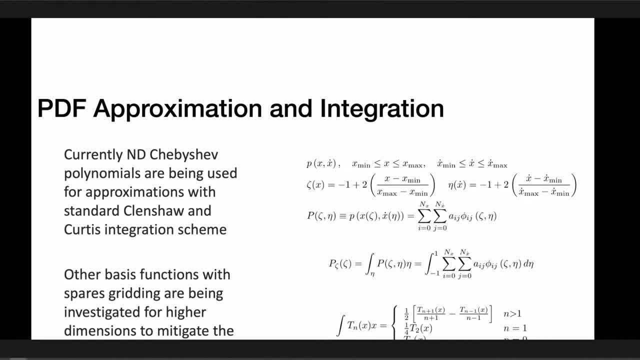 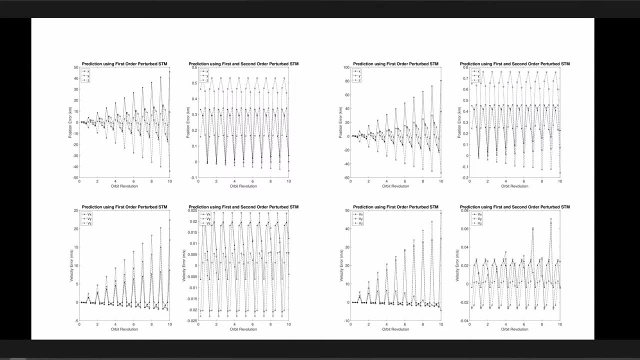 which is cannot be captured by by this. So, for example, in the drag case, there is uncertainty in the drag coefficient, which does exist. Then we need another way to approximate the, the uncertainty, because this business of uncertainty or handling uncertainty using the state transition matrix, as is shown. 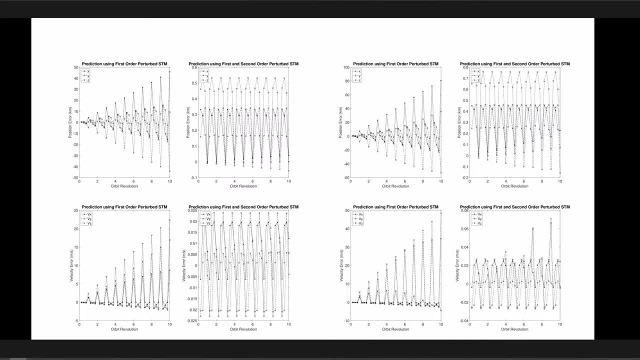 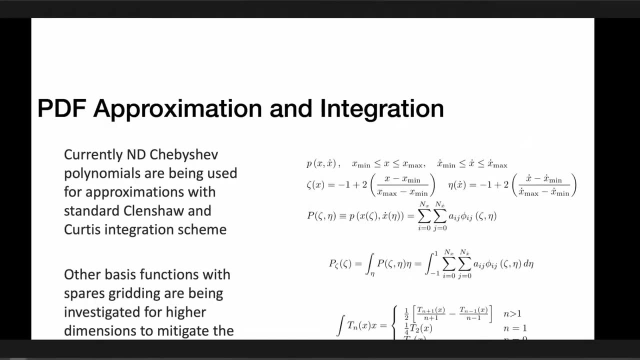 or, as is in the name, it is based on the state. It's a mapping of the initial state to a target or a final state. So uncertainty in the states gets mapped, but uncertainties in the parameters need a different approach. So you can create a sensitivity matrix. 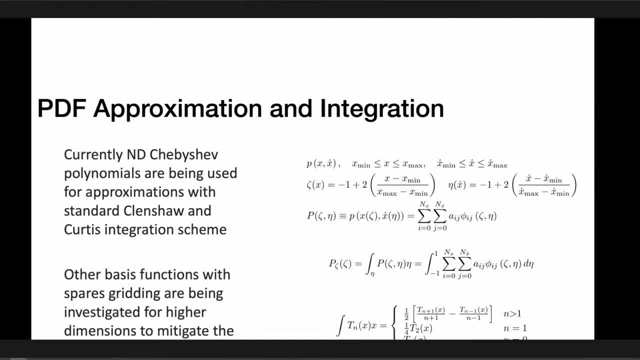 Another sensitivity matrix to parameters. but we went with another approach where we are essentially trying to approximate the PDF, the probability density function. So if you have the approximation of or you can obtain the approximation of the PDF, then you have a description of an analytic approximation. 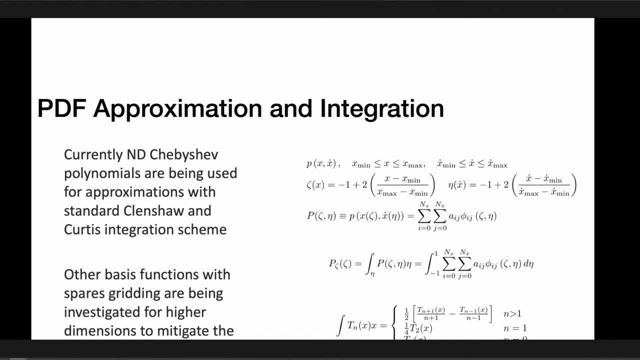 Then you have a description of the uncertainty surrounding any random variable. Now in the common filter, there is an assumption that these uncertainties remain Gaussian. Obviously, in real life this is not true. And as you increase the the observation times, or as you increase the propagation time, 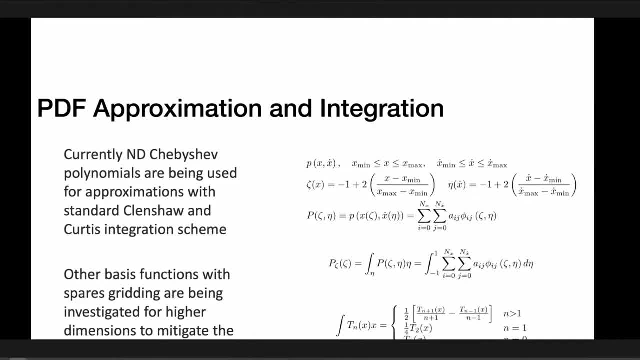 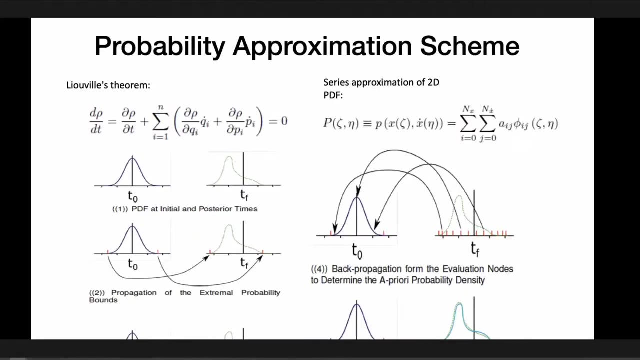 then these uncertainties become less and less Gaussian, as we have seen in the initial orbit distribution problem, where it goes all around the distribution. from a small sphere It becomes this distributed shape surrounding the whole, basically the whole original world. So our idea here is very simple. 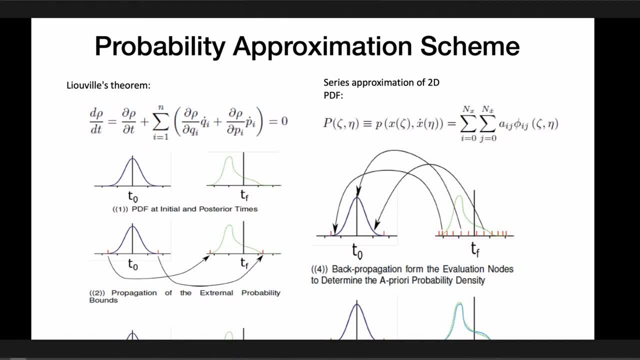 is that we're using the fact that we're using an aspect of Louisville's theorem that if the system is Hamiltonian, then the values of the uncertainties remain constant. So, or the PDF values remain constant, So, even if you propagate forward in time. 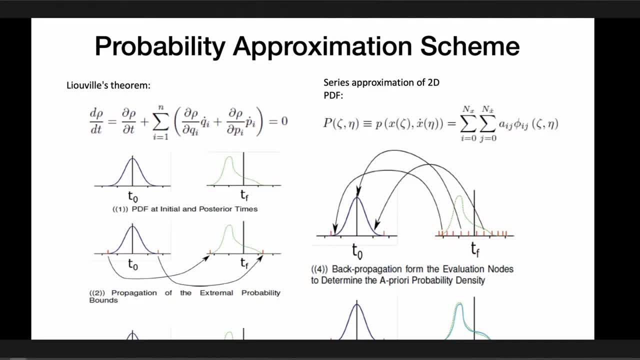 that these points forward in time. if you know what the original values are at the initial time, which you should know, you know, you know something about the initial distribution. This can come from the filter, For example, if you're applying a filter. 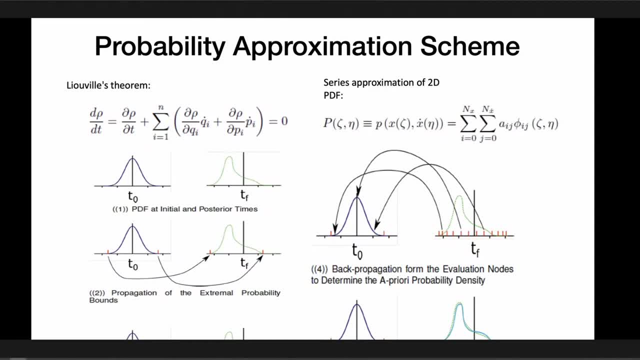 then it will give you an idea about what is the original distribution. Then you can essentially turn off the filter, propagate forward in time and essentially try to look at or try to approximate the uncertainty. So, because of this Hamiltonian nature of the problem, 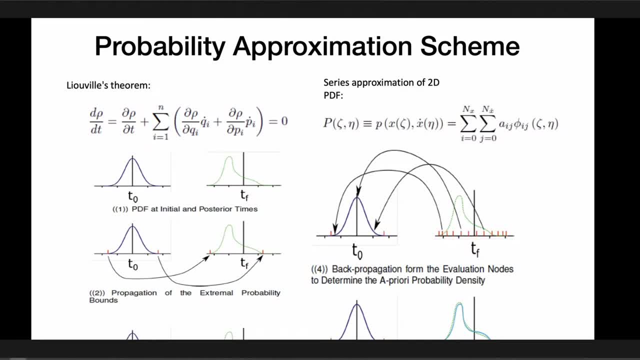 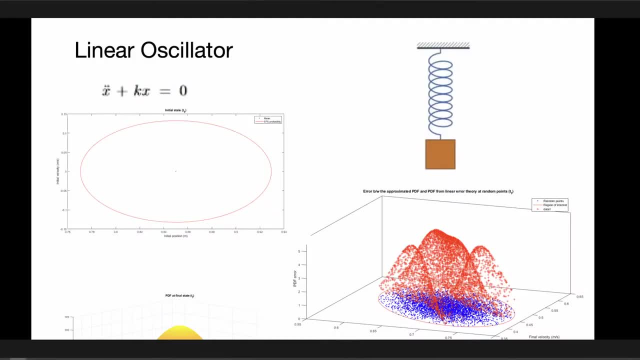 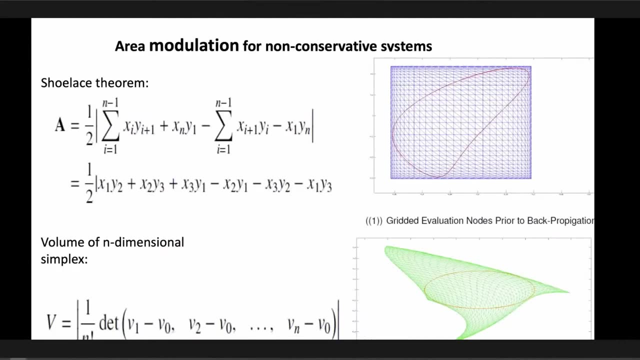 we can do this And we also address the non-Hamiltonian, non-conservative system of nature of the problem as well. So these are some simple problems to show the applicability of the method on the linear oscillator And this is how we essentially handled changes in volume or changes in area. 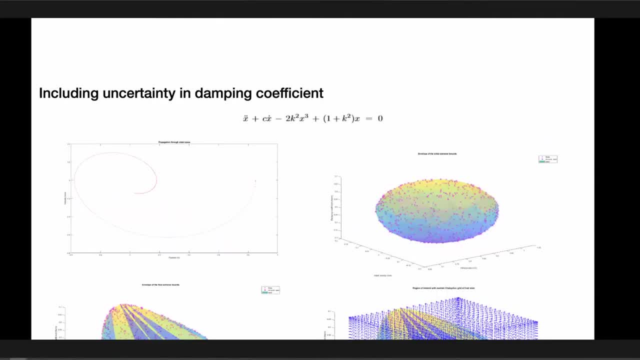 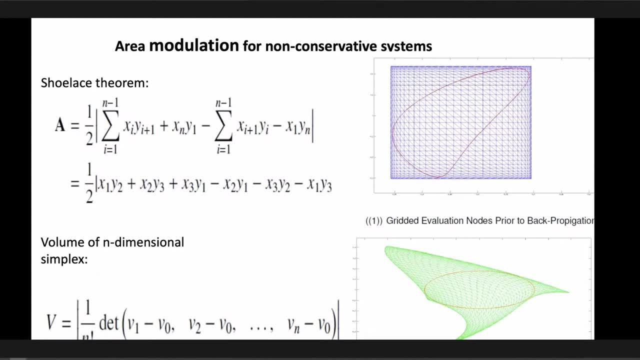 So what we did is trying to find- yeah, here's what we did, So I'll show you this in a few slides. But what we essentially did is we looked at the volume and then dimension and we came up with a scaling parameter that scales the original values to newly updated values of a certain scale. 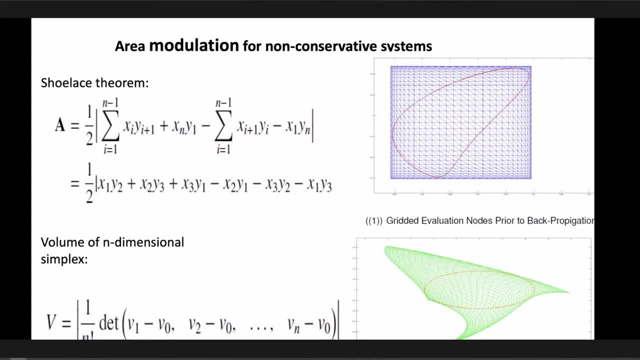 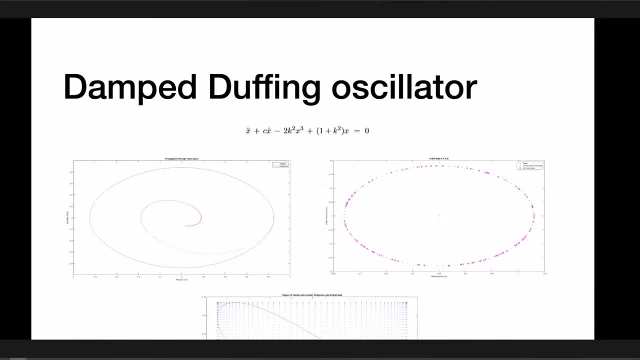 And we have done this scale locally, across the distribution or across the various levels of the nodes. So here we're showing the damping or the damp-duffing, And you can see now that the original, what is known as an original Gaussian. 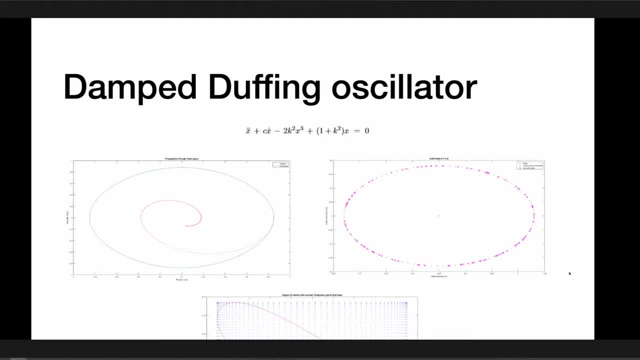 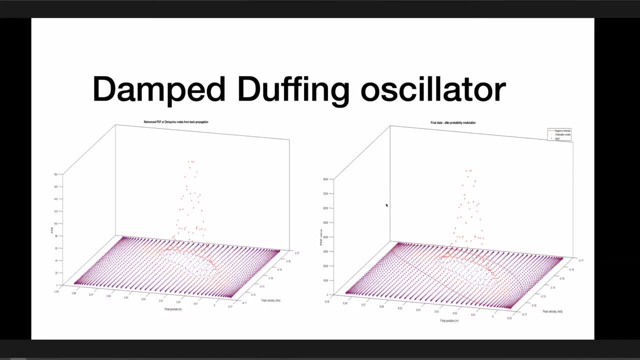 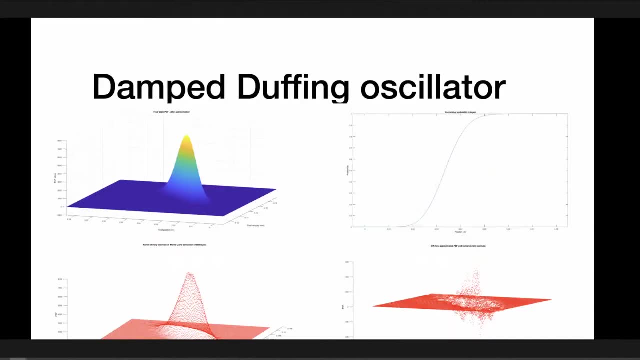 is becoming something that is not. this is not a Gaussian distribution, So- and you can see here that this is the trajectory of the damped oscillator- This is the probability distribution, And here we're using a couple of approaches to validate. One of them is that the property of the probability density function is that the total integral has to be. 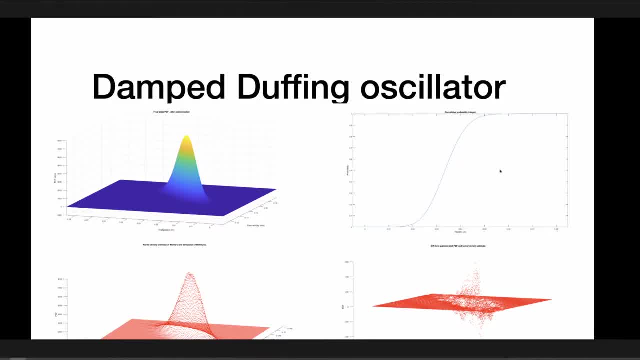 or the cumulative integral has to be equal to one. So here we're showing the cumulative integral to be close to one, which gives us confidence in the application. This is the approximation that we come up with Now here, and this is where the problem comes in play. 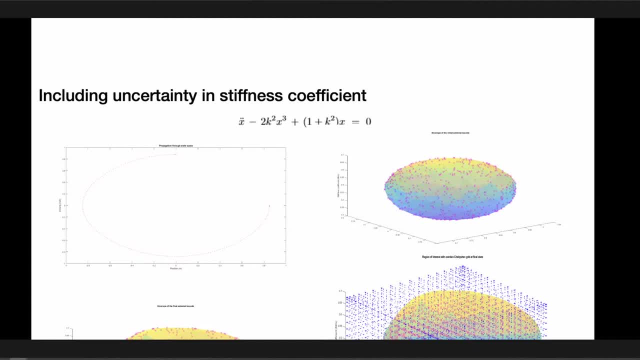 is that we are now including uncertainties in the parameters, So not only uncertainties that are related to the states, the initial states, as we did with the state transition matrix, but here we are introducing uncertainties in the k, in the stiffness coefficient, And now it becomes a 3D problem. 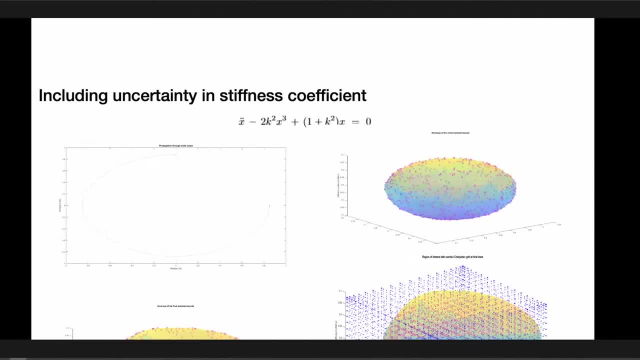 And this is how we deal with 3D problems. And you now have a 3D approximation technique where we find points on the boundaries of that shape. propagate them forward, come up with the approximation, propagate backward, find their values inside that ellipsoid. 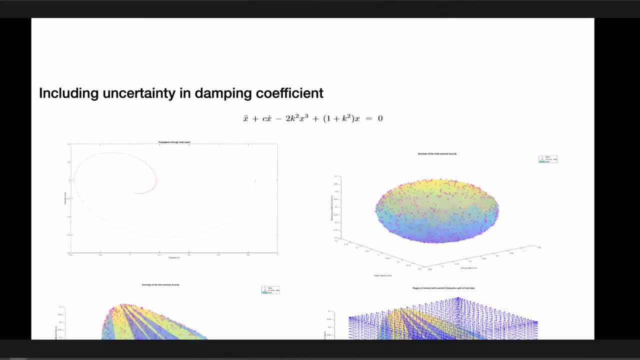 In this case it's 3D, And then we add uncertainty in that coefficient or the damping coefficient. So here we're showing. what we're showing here is that this method can actually be applied to not only state parameters, but also. 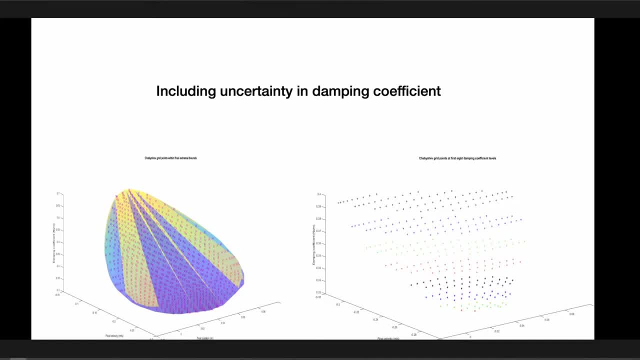 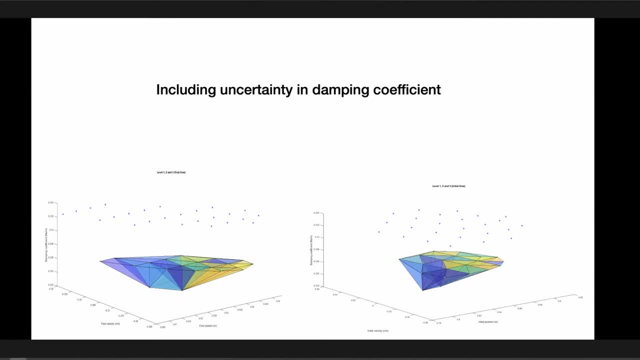 or state variables, but also system parameters. So here this is the method that we are using to modulate or to scale the volume, And you can see here on the left hand side, this is where we have the initial- sorry, the. 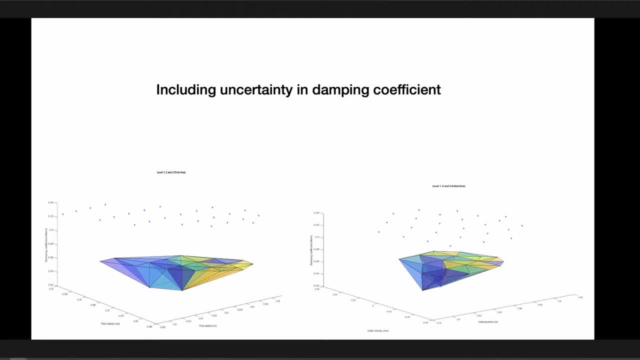 yeah, we have the final, the final time and the initial time And essentially we are approximating or coming up with the volume, the difference in volume or scale factor between the connected nodes. So this looks like more finite elements and tetrahedrals. 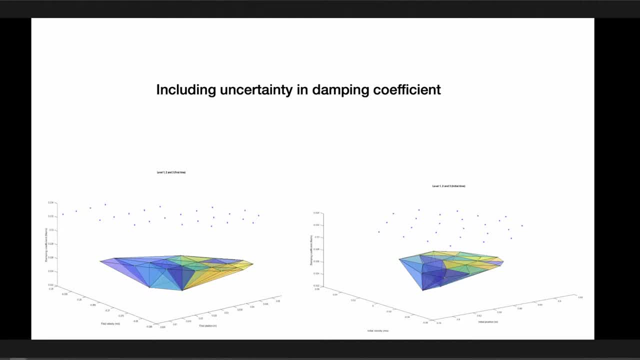 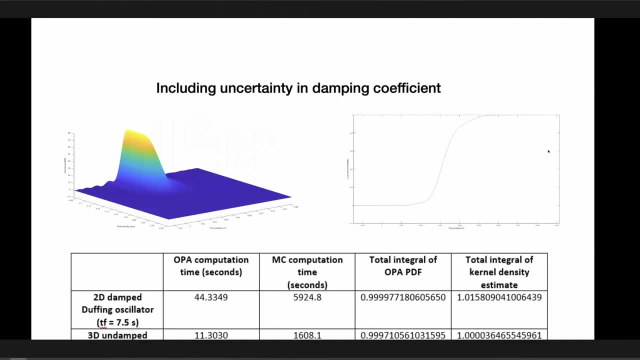 but this is essentially a way that we use, using approximation methods, to come up with the, with a way to find what happened due to the volume change, And here this is the most or a very significant time. A very, very significant result is terms of not only the accuracy, 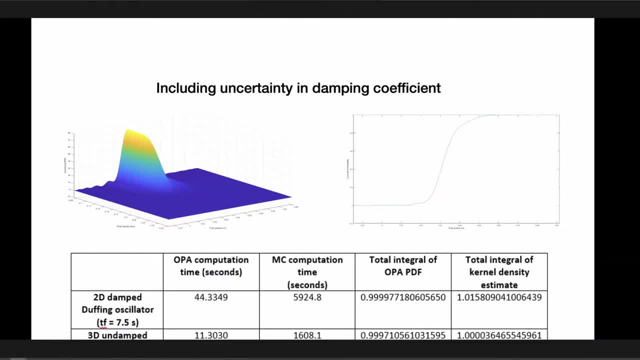 but also the computational cost of these methods, And we actually have improved over this even further. but this also shows you that we are talking about two to three orders of magnitude improvement. This is, we're talking about a hundred to a thousand times faster simulation than what you can do with Monte Carlo. 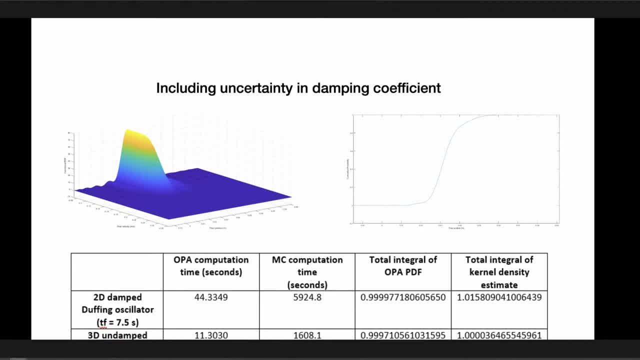 Now Monte Carlo, the way you go if you want to do a high fit again. this is high fidelity approximations. We're not talking about back of the envelope kind of thing that gives you a quick result. We're talking about high fidelity accuracy. 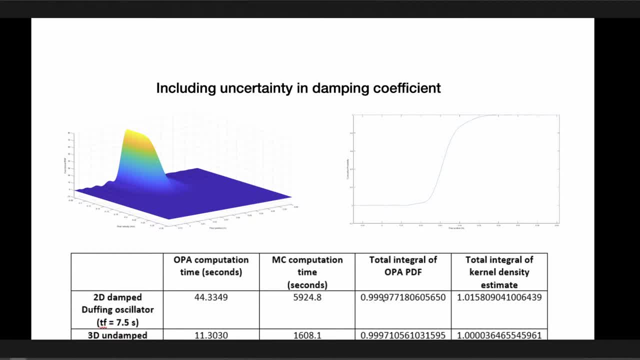 So we're talking about an integral that is accurate up to four to six digits, which requires Monte Carlo to run for millions and millions of coins for 100 to 1000 times more time than this approach. So this approach lends itself very nicely to. 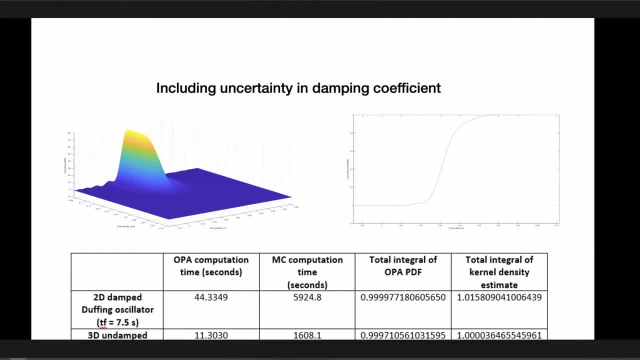 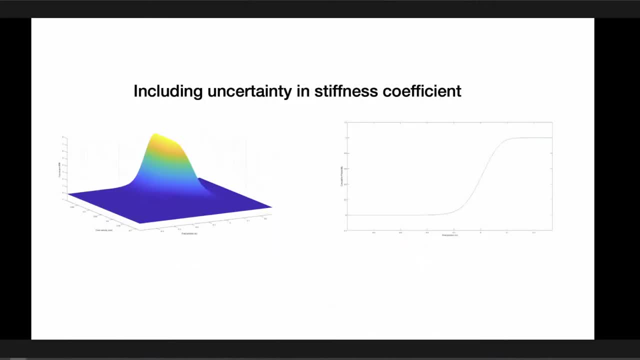 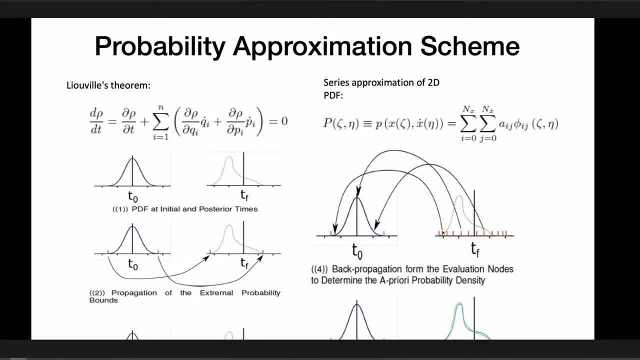 to reducing the computational cost and improving- and while still producing- very high fidelity- results. Other aspect of this approach is that it's highly parallelizable. You see here, once you start distributing or creating these nodes, you can essentially create a parallel process to back propagate or to propagate these points back in time. 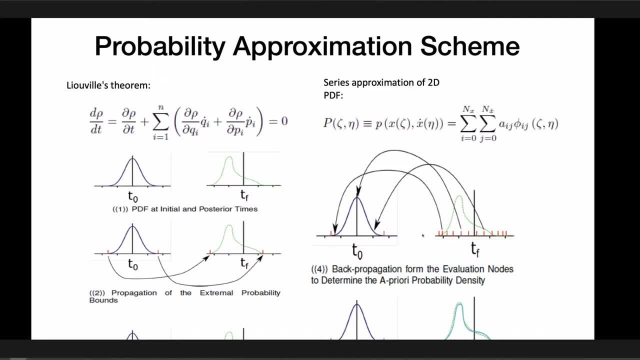 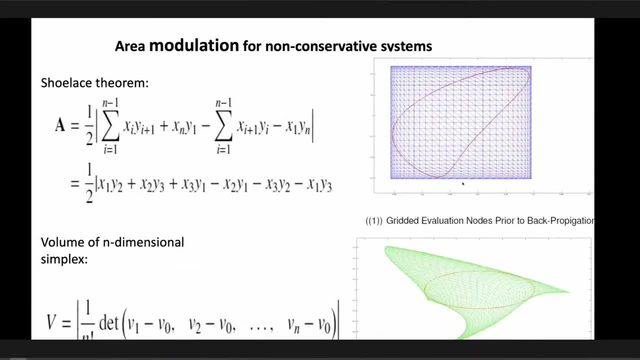 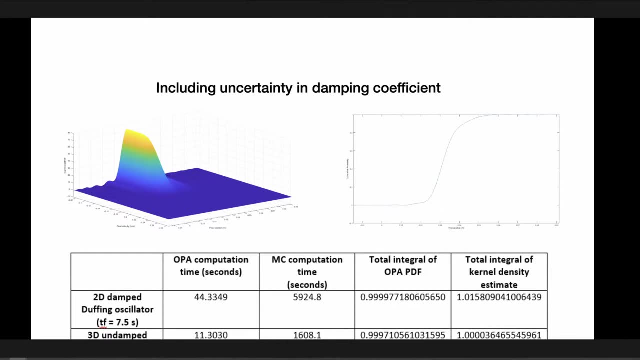 and find their values separately, because they are all decoupled. They are just distribution of nodes or a selection of nodes that we had came up with. So, even without parallelization, we're talking about this much accuracy and we can do the same thing with parallelization. 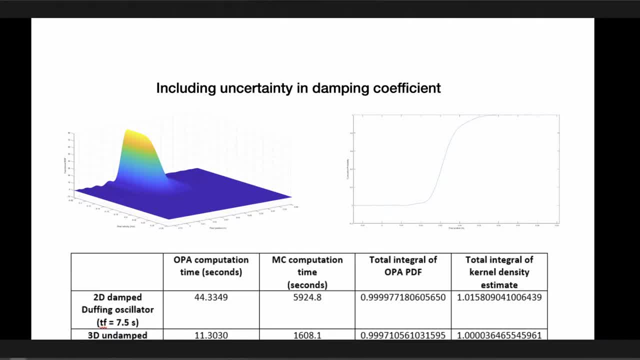 I think it. I believe that it will maintain the same level of accuracy and it will be more hardware implementation amenable than Monte Carlo. So even if you were able to or you can, parallelize Monte Carlo, but still the difference here we're talking about 100 to 1000 times faster. 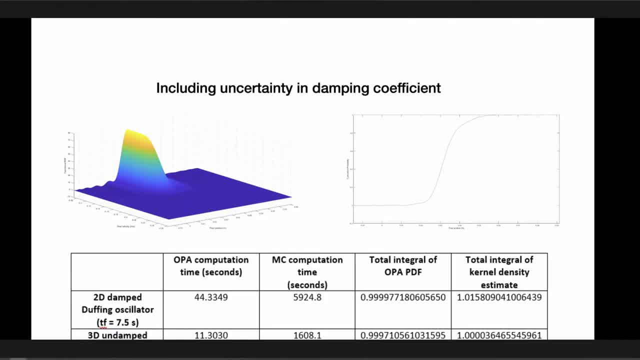 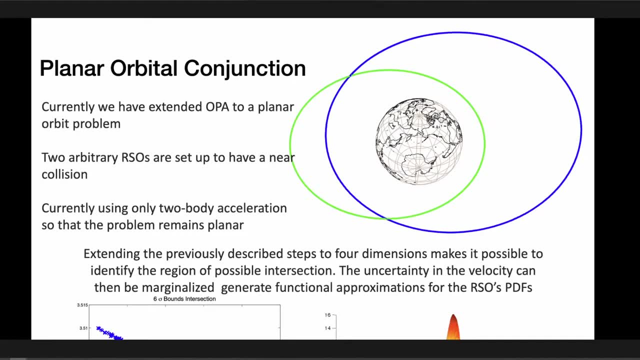 So with parallelization we're talking about stuff that can actually be implemented on hardware, and not just a supercomputer or a desktop computer in this case. So we move in, we move into the orbit problem and we're using the same techniques. The orbit problem is. 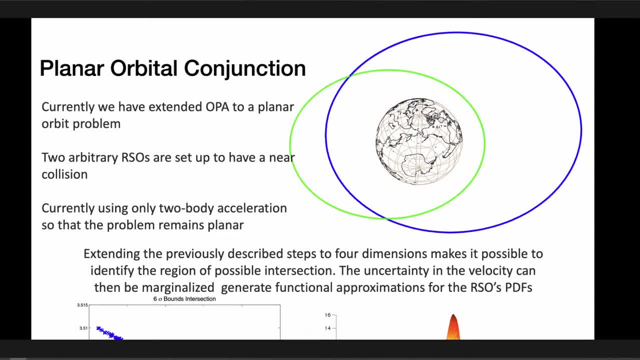 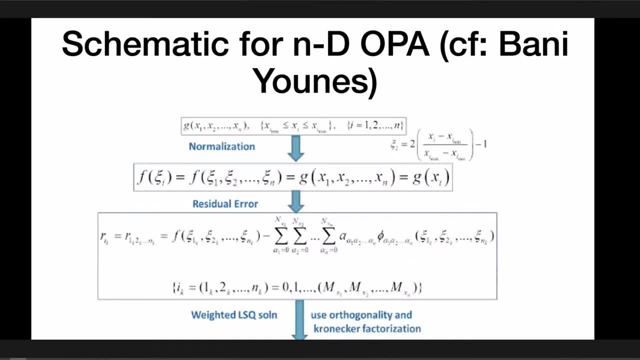 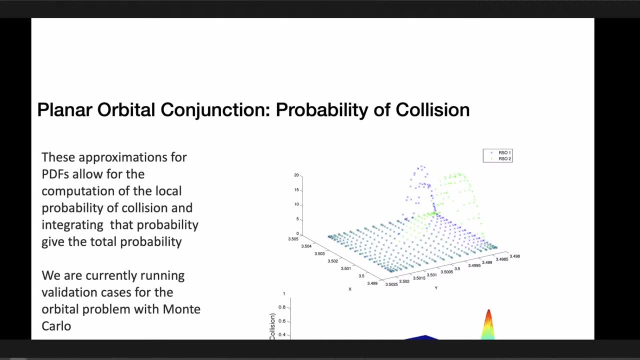 is more nuanced because now it becomes a four-dimensional problem in the uncertainty domain. So once we have this, we can essentially look at the overlapping of the two PDFs. And if we look at this overlap, what we can do is that we can accurately compute the probability of collision between two objects in space via 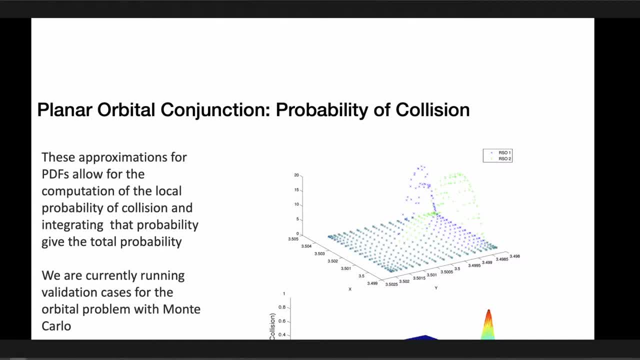 via analytical relationships, via analytical or mathematical expression. We don't have to do Monte Carlo and count points and do all this kind of stuff. We can actually integrate in closed form and come up with an accurate number. Now we're actually currently we're working on validating this with real data to see if our prediction can encompass what a real satellite does. 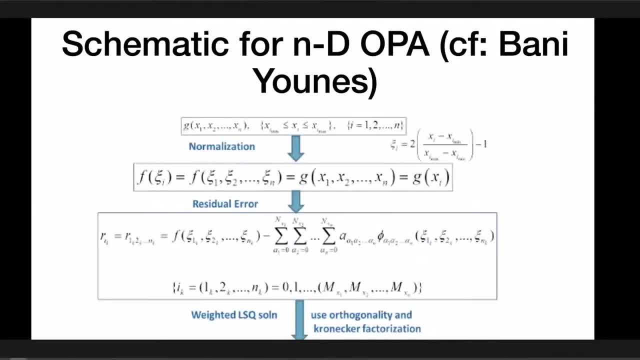 And hopefully we will be able to validate this very soon Now. this work can also be expanded to higher order, And this is some flow chart that shows that the same idea that we use for 1D, 2D, 3D and 4D can expand it to ND approximations. 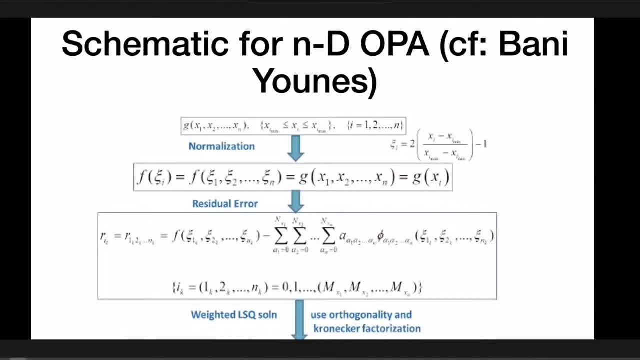 And this is from our colleague of mine that in my group when I was doing my PhD, So he published this and we're also studying this to expand our method to higher dimensions beyond ND. So this is most of my talk today about astrodynamics. 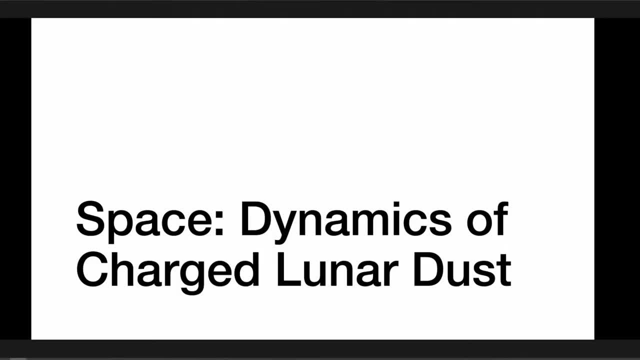 And this is a main area of research. I'm going to go quickly over some research or another very, very significant area that we're working on, And I know I'm running out of time So I'll do this very quickly. We're also exploring dynamics of charged lunar dust. 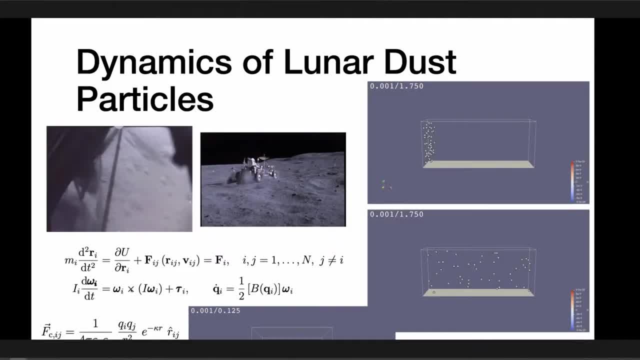 And what I'm showing here- and this is where the connection of this whole research, the three circles that I showed earlier- is that this is a nonlinear, dynamical problem, very similar to the orbit problem, to the multi or the N dimension or the N body problem. 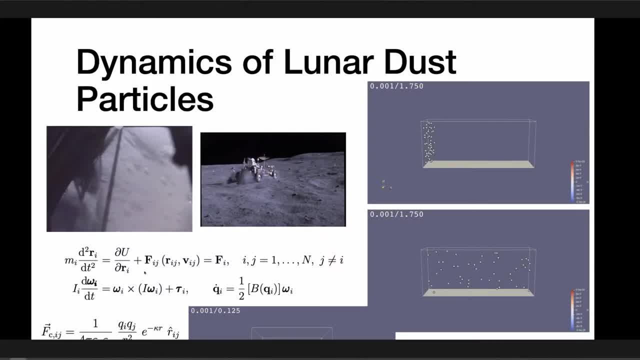 if you will, You can represent N number of particles as an N body problem or a multi body problem, And what we're trying to solve here is that existence of of lunar dust hanging on the lunar surface due to the rover moving on the surface. 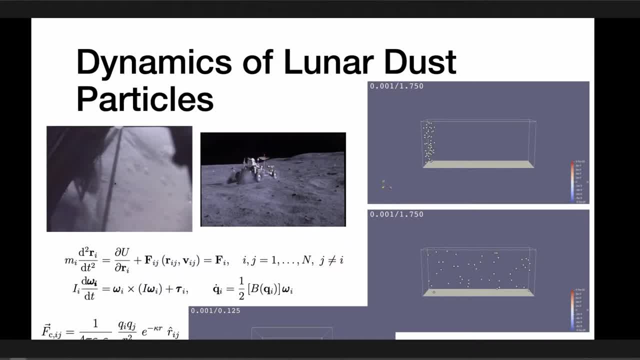 Due to landing and taking off, due to moving of the motion of astronauts on the surface or any perturbation, natural or man-made. Now one could say that this is an actual phenomenon. It happens on Earth, It happens everywhere else. 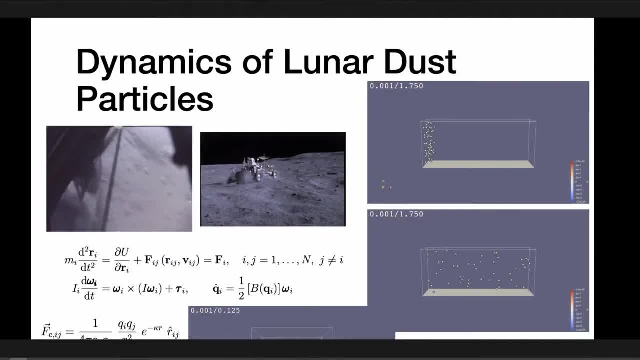 The difference is, as you all know, the moon has no atmosphere, It's in vacuum. So if the dust particles are not moving due to their ballistics or free fall without any, any other factors, then the formation of these clouds and the motion of these clouds on the lunar 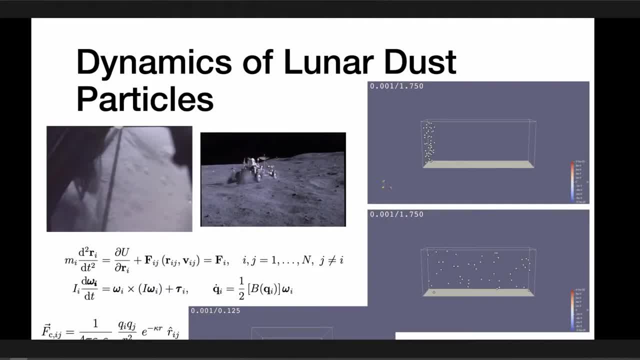 surface has to be explained via something else, Not like here, like dust particles hanging in with the atmosphere. So what? what we? the prevailing hypothesis is related to lunar dust charging or electrostatics, And we have been conducting several numerical experiments to look into this phenomenon. 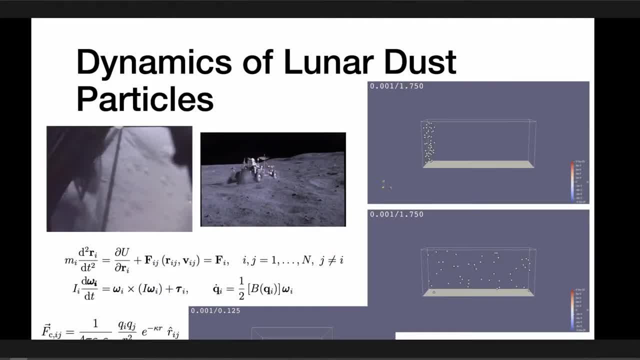 try to understand it and try to understand how these dust particles behave. So these are some videos, but I don't have time. but you can see, here we're looking at several particles that- and I think this one is faster- So several particles that have a positive and negative charge. 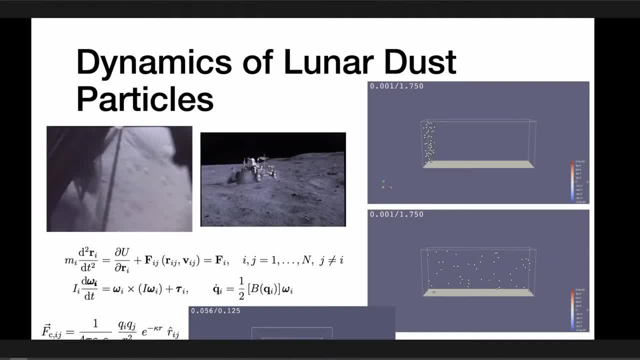 and you can see how the, the, the, the affect each other and how they essentially get attracted and repel each other in in that, in that domain or in that space. So we're looking at these simulations to understand how the dust form and move due to electrostatic. 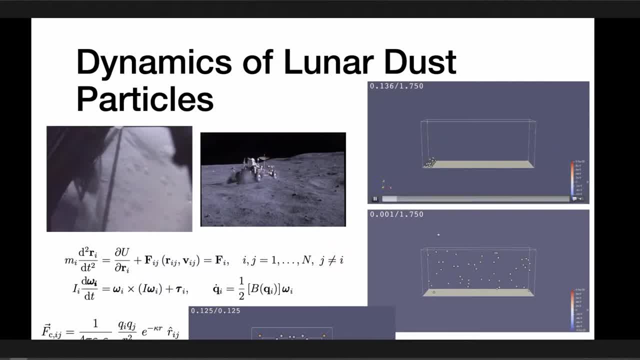 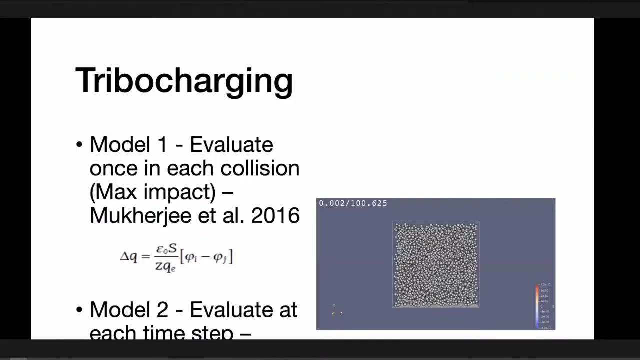 charging- The other area that is very interesting, Yeah, and these are the various simulations that we have been running. So these are typical experiments that are done in this area, where you slide particles on on a surface and you compute the interactions. So 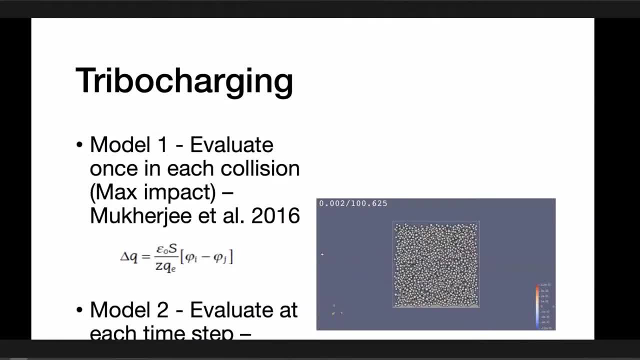 one other area- and I know this is very brief and it doesn't give this work its justice, but we don't have a lot of time, So I know that. the other area is that we're not only. it is related to these charge. 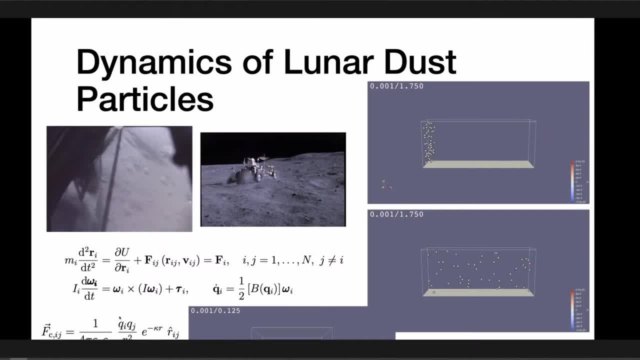 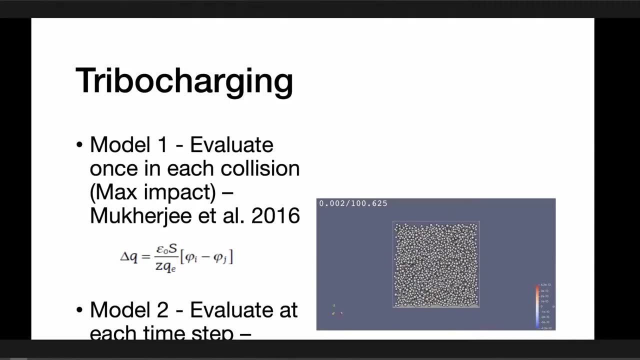 these forces coming from the electric, electrostatic forces, coming from the chart, the particles having charges on them. It also comes from tribal charging where, essentially, tribal charging is essentially the phenomenon, that charge is being transferred from one particle to the other via contact. Think of 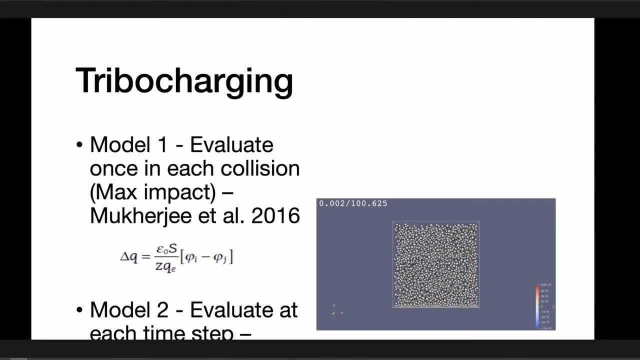 you know, having a pen or a pencil and you rub it in your hair and you pick something up. So this is electrical Electrostatics, So you can think of these things. So we're looking at model-based approaches and you can see here. 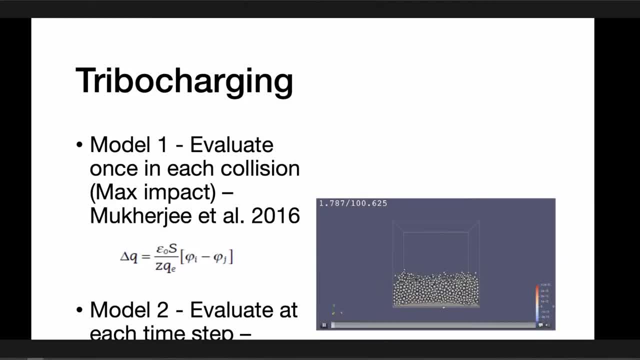 This is a another famous experiment that we validated using discrete element methods and essentially by vibrating that with particles having interaction, mechanical, obviously, interaction due to the vibrations and obviously they get charged because of all the friction And all the contact and you start seeing, you know. 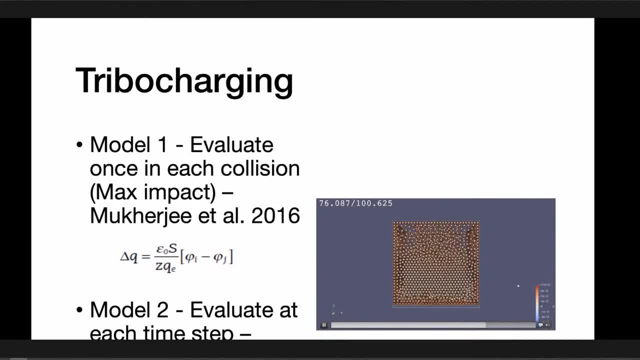 the behavior of these particles due to tribal charging. So this is another experiment that we're looking at Now. we have looked into, we have went way beyond these elementary results and we looked into how does lunar dust itself behave and in the lunar environment, using the appropriate gravity. 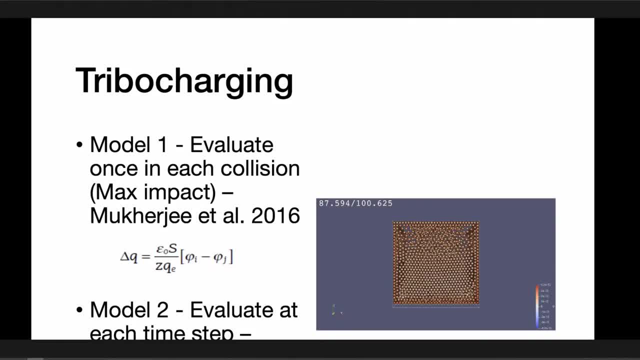 the appropriate electric fields, the appropriate values, values for the particles. and what we have found- and I don't, unfortunately, have a slide to show that here, But what we have found is that there is the electrostatic do affect the electrostatic forces, do affect the lunar. 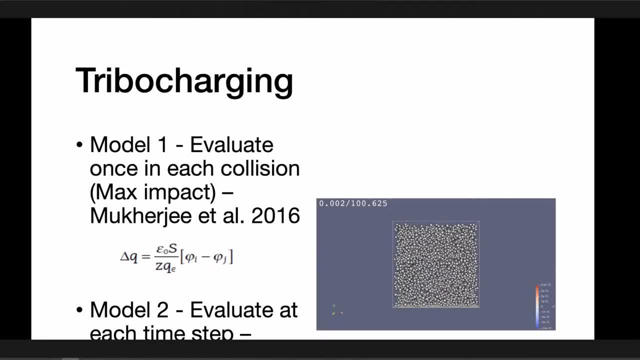 the lunar dust dispersion and the cloud forming of the lunar dust quite significantly, And we have some sensitivity analysis that shows that and also some preliminary results that show that the dispersion is several orders of magnitude In terms of the, in terms of from the inertial or the inner initial distribution. 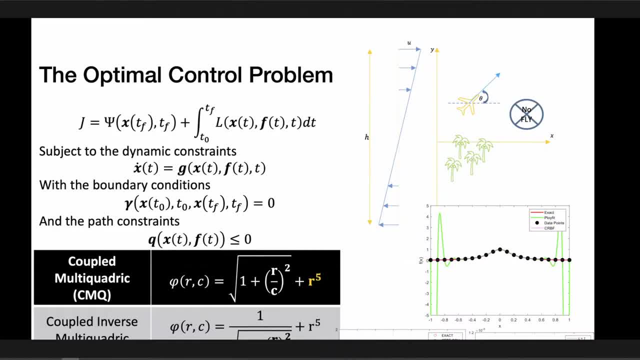 Quickly over controls and robotics. We're looking at optimal control problems, guidance in in an environment that has obstacles, and changing. We're looking in some computational techniques to do this. And finally, this is the robotics portion of the lab. And finally, this is the robotics portion of the lab. 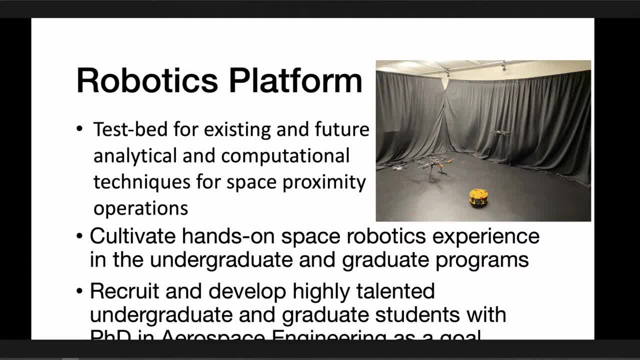 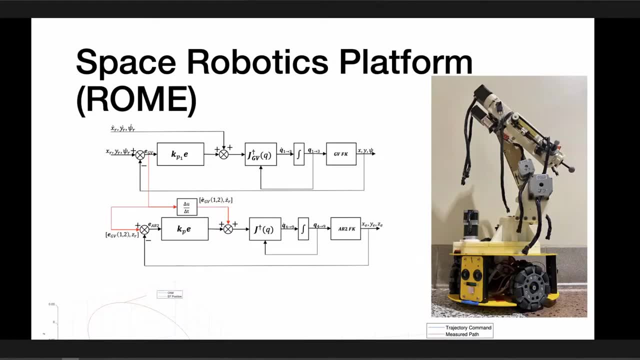 And finally, this is the robotics portion of the lab. We have several UVs, several ground vehicles. We're doing experiments that implement some of the control, or we're planning some experiments to implement some of the control schemes that we develop, as well as experiments that uses this platform. 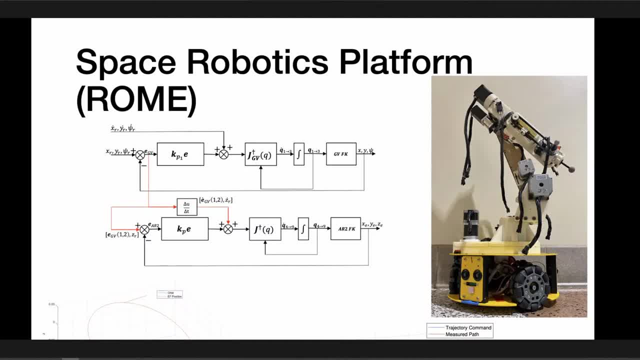 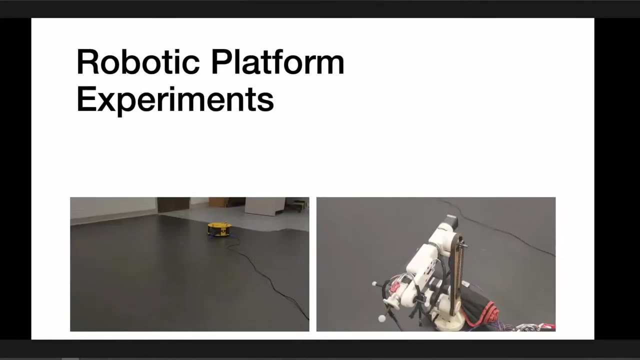 which we call Rome, and basically try to emulate space motion. This has good applications in sensing and and also to show the orbit motion As we see here. these are experimental results from the kinematics model And now we have a dynamics model and the group has been working very actively in this area. 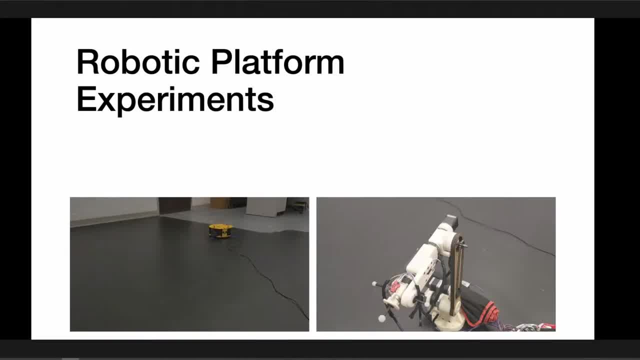 Here are some videos for the, for the ground vehicle doing a circle, And it's very loud. but- and this is the motion that we can produce with our robotic arm- We now have a new robotic arm that can essentially produce More smooth or smoother dynamics than this. 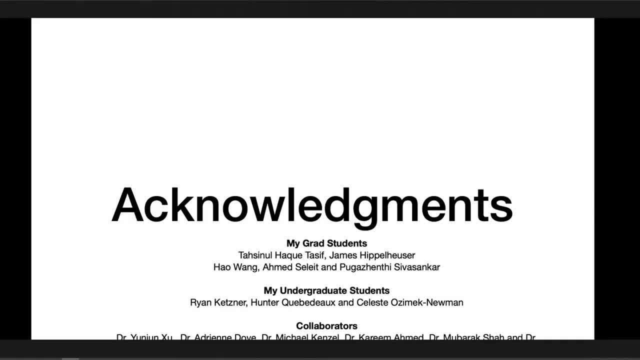 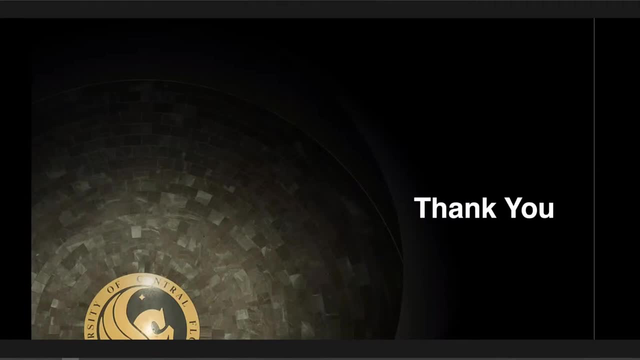 Sorry, I went a little bit over, So I'd like to acknowledge all the graduate students in my group- Most of them are here. Thank you for being here- and also undergraduate student researchers, collaborators and funding. and thank you and be happy to take any questions. 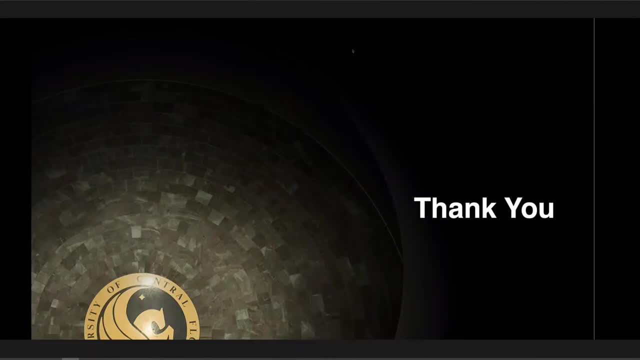 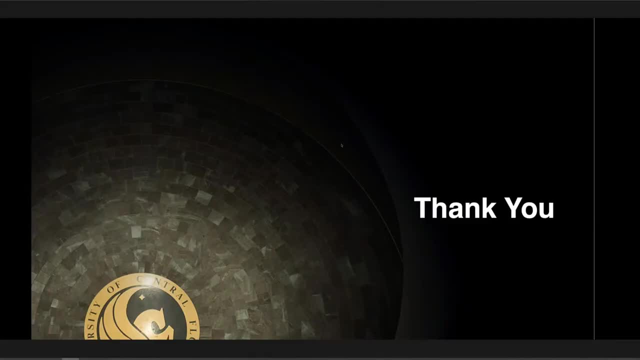 yeah, it's been a while since i took astrodynamics, so it's kind of took it a second to come back to me in the middle of the presentation. okay, i'm glad it's always good to keep these things going. keep the memory fresh, all right. all right, i don't see any questions. um, yeah, thank you so much for coming tonight. 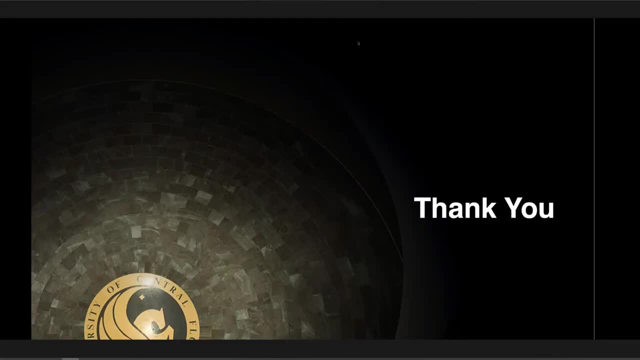 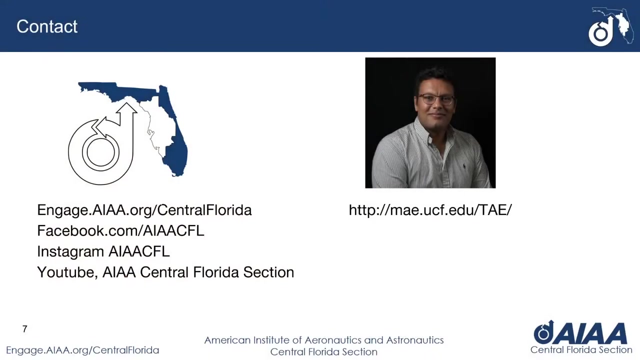 thank you. yeah, it was really exciting to see what you guys are working on and all your students there in the lab. thank you all. right. so, yeah, thank you all and i hope this has been insightful. and uh, yeah, hopefully we can do more more of these talks in in the near future. 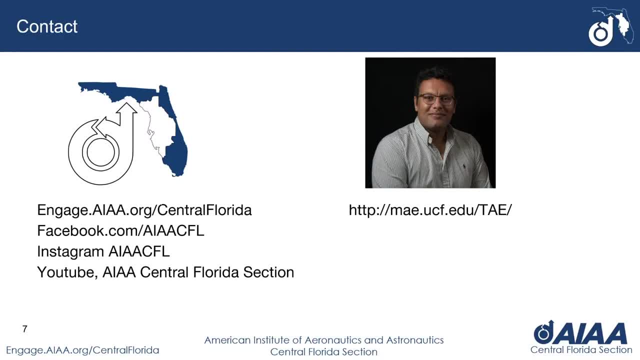 maybe i can't dedicate another talk about the lunar dust problem and another talk about the controlling robotics problems that we're looking in. yeah, that sounds great. um, yeah, we're also allowed to have your students as well, if any of them- yeah, yeah, graduate or undergraduate this time. yeah, this time around they can do a better job in focusing on their areas. 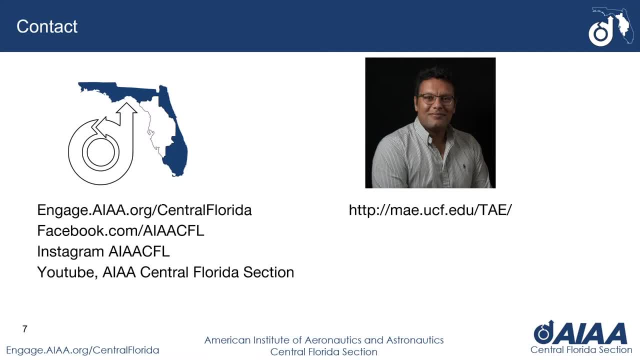 than what i, what i would be able to do. yeah, it'd be great to see what those guys are working on. yeah, sounds great. yeah, thank you. have a good evening everybody, you too, thank you bye. yeah, well, thank you to dr algohari for a great presentation. 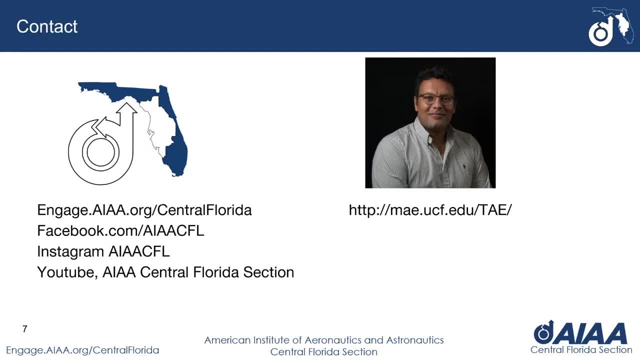 and if you guys have any questions for him, his website is on the page here, maeucfedu. you can also contact him. his email address is on there on their faculty page at ucfedu for aaa, central florida section. if you have any questions or 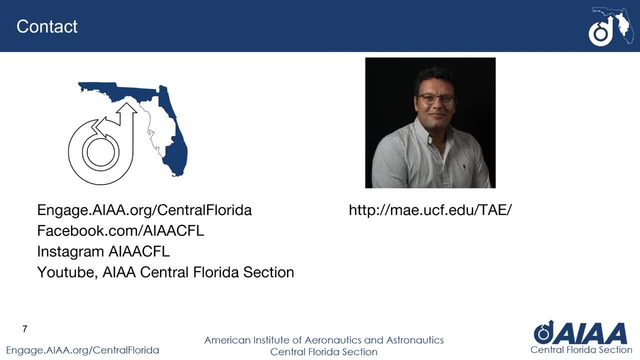 potential speakers you'd like to see in the future, cool ideas for events like this. we're always open to new ideas. we love to have speakers as much as possible about a variety of different subjects and areas of study. so if you have any questions about a variety of different subjects and areas of study, so if you have any questions- 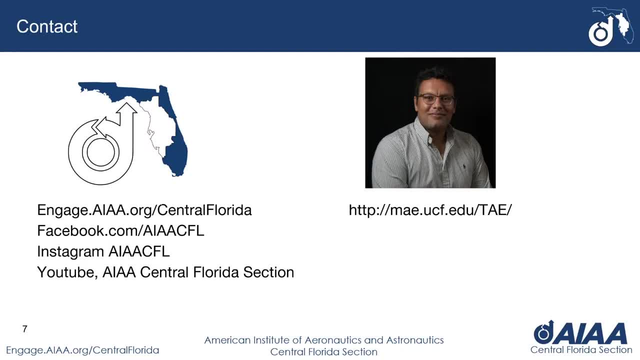 about a variety of different subjects and areas of study, so if you have any questions um so, you can contact us at aaacentralfl at gmailcom or at any of our pages here, like our facebook and instagram, or you can subscribe to our youtube channel to see more. 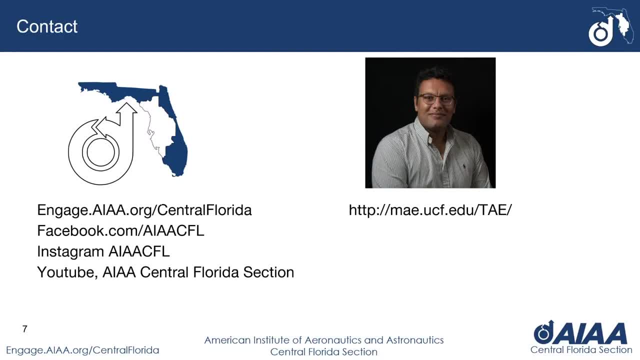 events like this and check out our previous events that we record. they're all available on our channel, usually the day after they go up, so if you can't make it that evening or that day when we host an event, you can always check it out on youtube later.